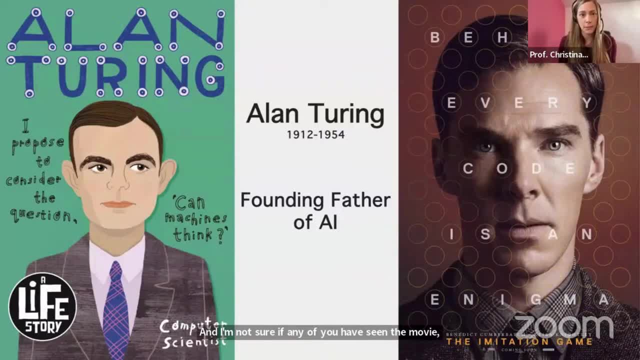 which I have here to the right, the movie called The Imitation Game. So The Imitation Game is based on all of his work that he did, And through his work, not just in the war but before that as well, he was the first person to start introducing the idea of algorithms and computing machines. 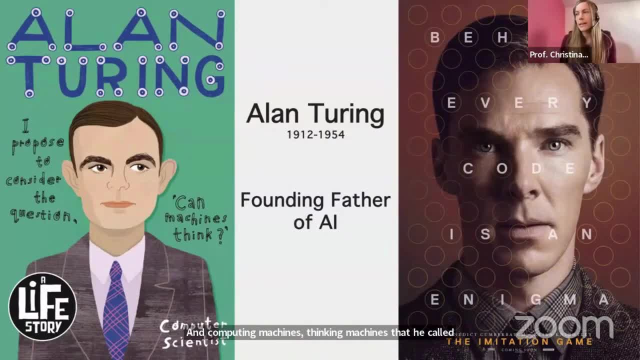 thinking machines that he called them. So he began and he's- he's- really considered the founding father of AI. Now I mentioned the movie The Imitation Game that you see here, pictured to the right. The Imitation Game, this name, this word is actually 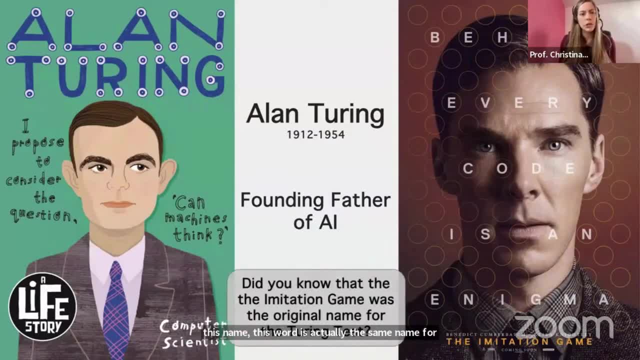 the same name for the Turing test. I'm not sure if the Turing test sounds familiar to you- Some of you it might others it might not- But I'll explain to you what is the Turing test. But keep in mind that The Imitation Game was actually the original name for the Turing test. 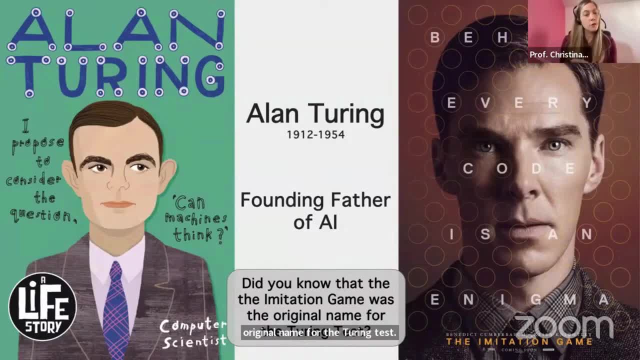 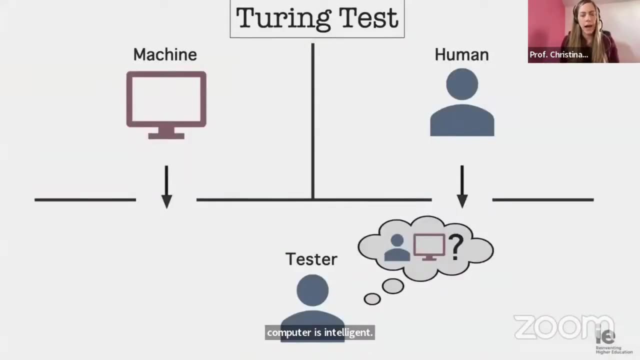 So what is the Turing test? The Turing test was, of course, created by Alan Turing, And this was a test that he decided to propose as a way to measure whether a computer is intelligent. So this is the way that it works. Here you have, like my diagram of how I would. 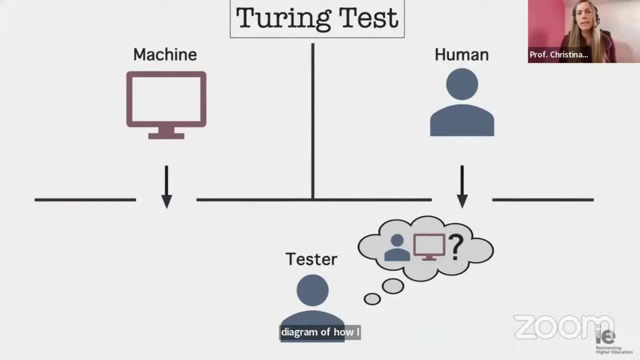 how. I would explain how it's working. So the Turing test is this test of a machine's ability to exhibit intelligent behavior- intelligent behavior that is indistinguishable from that of a human- And the way that it works is: you have this diagram here, So let's start at. 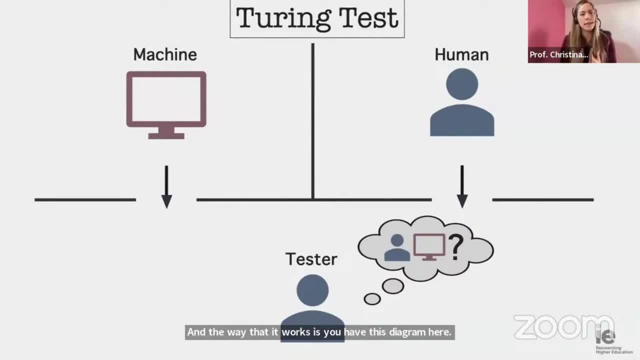 the bottom You have the tester or the human evaluator. We can say that I'm the tester And I would be chatting with both a machine and with another human, chatting through text only. You can imagine it like a chat bot And the tester myself I would be. I would be challenged. 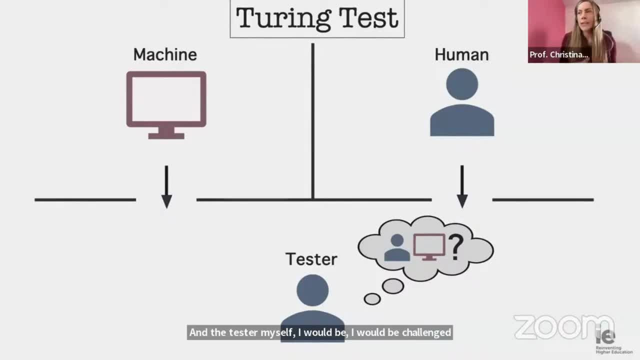 talking to both the machine and the human, challenged to try to determine which one is the machine and the human, And I would be talking to both the machine and the human. which one is the human? Can I tell the difference between them? And if the tester 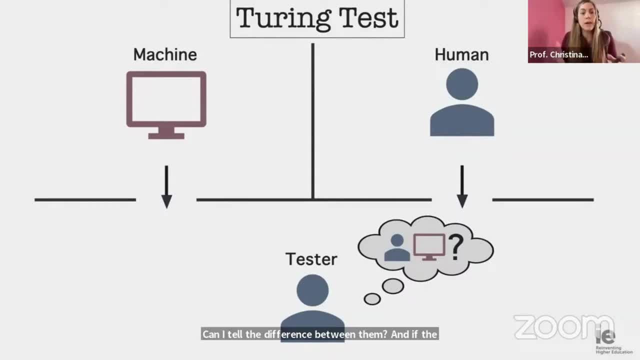 if I cannot reliably tell the difference between these two, if I can't tell the difference and decide which one is the machine, which one is the human- because the machine is able to trick me enough- then we can say that the machine has passed the test. They are exhibiting this human. 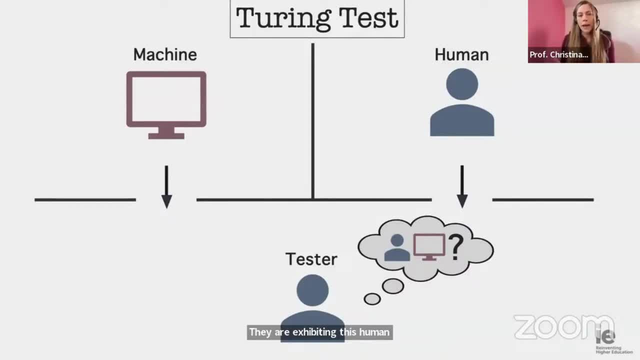 level of intelligence. Now, this was proposed by Alan Turing a long time ago, 40s and 50s- And it's been, it's been used now ever since as a great way to measure intelligence. But of course, it's true that 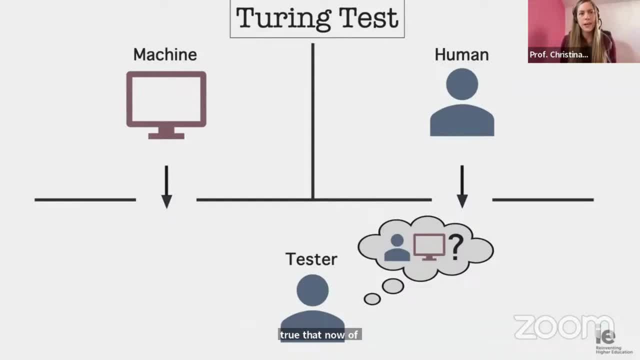 now, of course, with with ChatGPT, large language models, it might not be the best test anymore. ChatGPT is very, very good at chatting with us in a human like way, But it's still. this has lived around with us for many years Now. there's other ways to measure intelligence, Especially a lot of 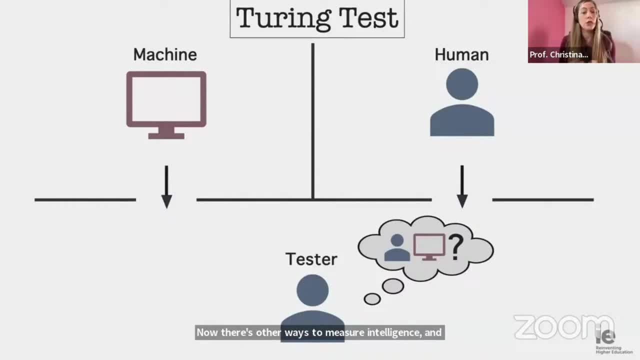 people argue that a really good way to measure intelligence is through strategy games or through video games, And I think that's a really good way to measure intelligence, And I think that's a really good way to measure intelligence And I think that's a really good way to measure intelligence. So you 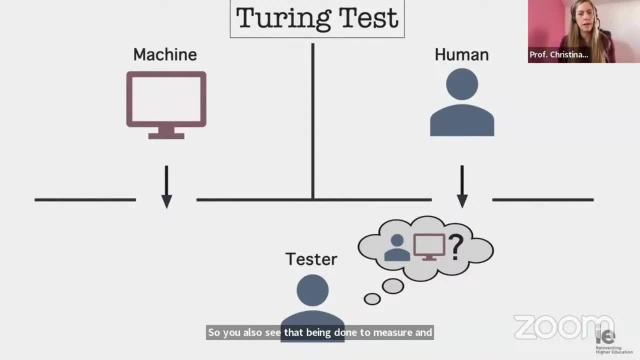 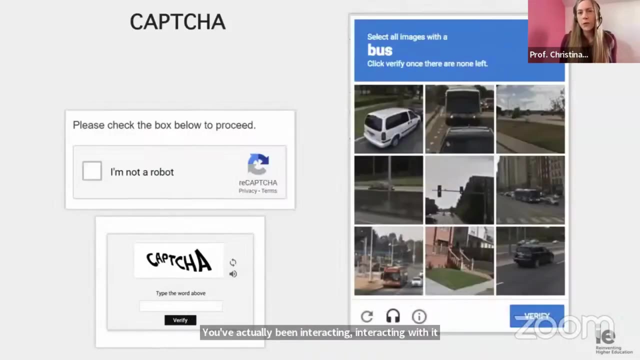 also see that being done to measure intelligence of machines. Now, I've mentioned that the Turing test began 40s, 50s, And what you might not realize is that the Turing test lives all around us. you've actually been interacting, interacting with it for years. Does anybody know what does? 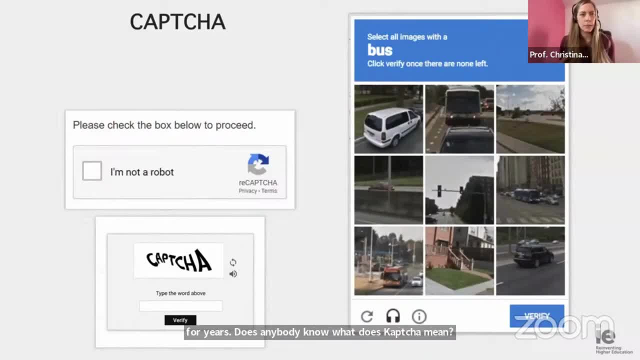 CAPTCHA mean. So I'm sure all of you are familiar with these images that you see here. we get them all the time when we go on on websites And this is called CAPTCHA. But I think what we're going to most people don't realize is what does CAPTCHA mean? So CAPTCHA is an acronym And it stands for. 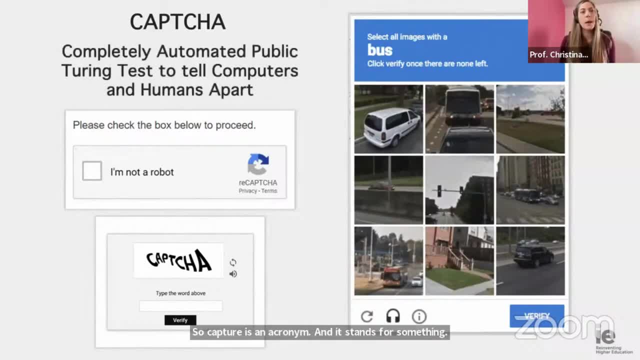 something It stands for: Completely Automated Public Turing Test to Tell Computers and Humans Apart. So you probably didn't realize it, but you've been interacting with a form of a Turing test all of these years when you've been navigating the web. Now, unfortunately, Alan Turing- he passed. 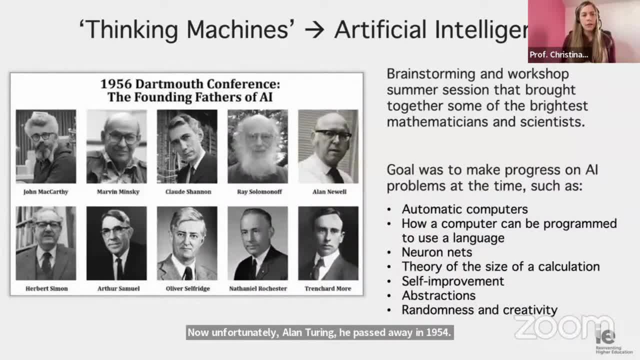 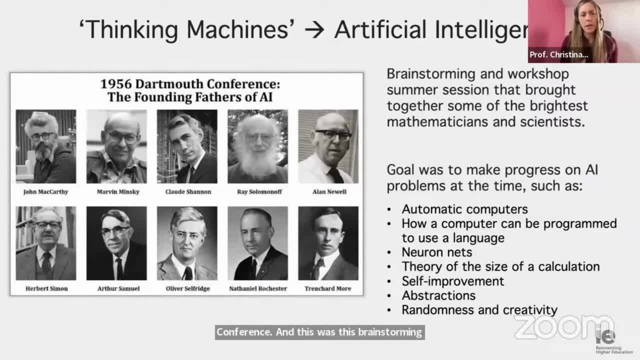 was this brainstorming and workshop summer session that brought together some of the brightest minds at the time, some of the brightest minds in mathematics, science, computers, etc. And they all met and spent a summer trying to crack some of the some of the hardest problems around AI. 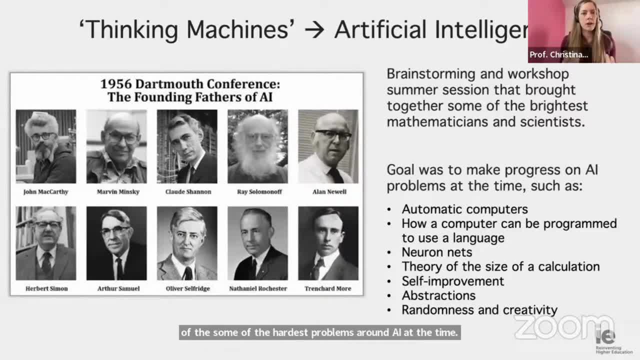 at the time. So things like you can see listed here: automatic computers, how a computer can be programmed to use a language, neural nets, which is the equivalent of neural networks- it's a type of algorithm that we use today- And even things like randomness and creativity. So all of these. 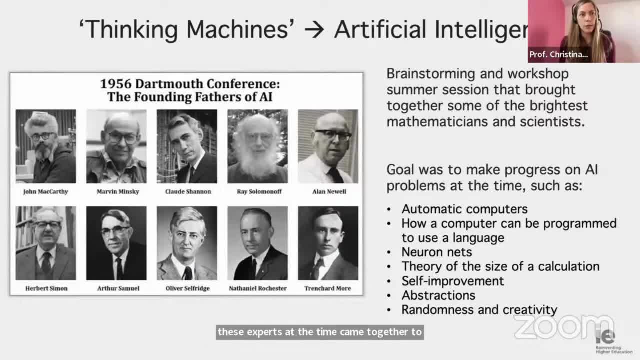 these experts at the time came together to try to crack problems around what was originally called thinking machines. Now, around this time as well, this was the moment that they coined the term artificial intelligence, So before that it was called thinking machines by Alan Turing. Later we 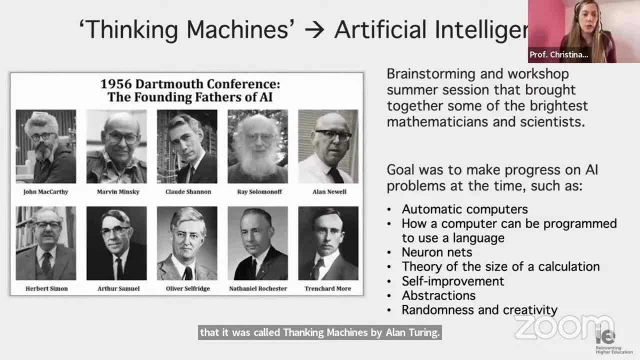 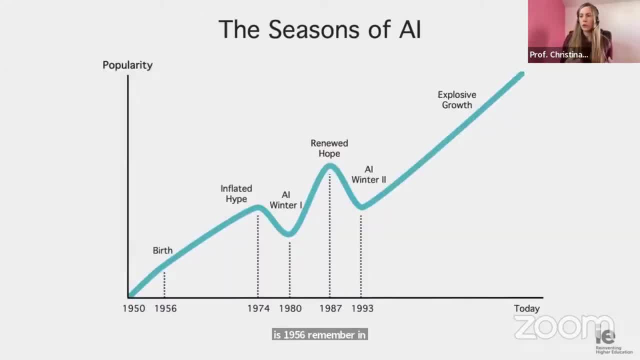 finally gave it the name artificial intelligence, which is what we use still today. So this is 1956.. Remember 1954, 1950s, 40s. Alan Turing began with everything, So we can call this the birth of AI. 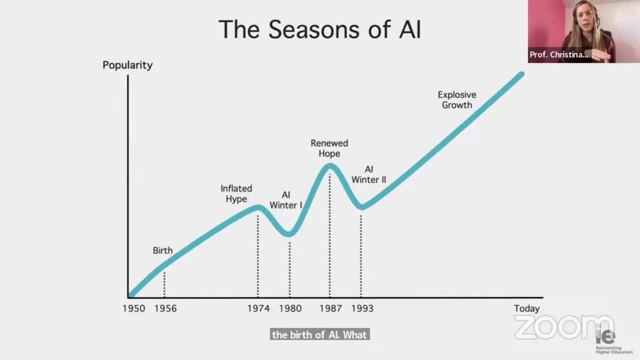 What you're seeing here you see on the horizontal axis, on the bottom you see over time, and on the vertical axis you see the Earth, And then you can see here: this is the popularity or the usage of AI. So we're looking at the popularity and the use of AI over time And you can see here. the birth of AI that we've just spoken about began in the 1940s, 1950s And then ever since then, AI has followed what I like to call the seasons of AI, And you can see here how it tends to go up and it goes to a peak and then it falls back down And then it goes back up again and then falls back down. So the 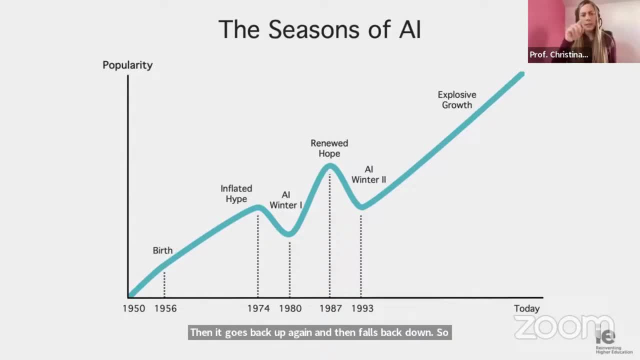 it goes through these cycles And these peaks. these peaks are what we would call like inflated hype, that everybody gets very. they have a lot of hope and aspirations for AI. they think that we are, you know, on the on the edge of discovering something incredible. So we have this really, really growth in, in hype, And then what tends to happen- and it's happened twice before- is the hype doesn't live up to expectations And we fall into what is called an AI. 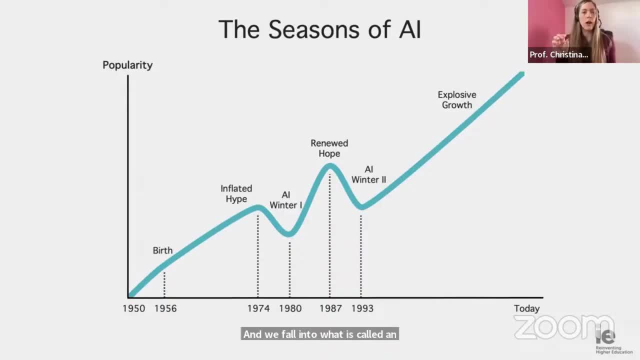 winter, the, these moments of a drop, a drop in the AI popularity and use. these are called AI winters, And this is a moment when AI hasn't hasn't really lived up to its expectations. people become disillusioned and you start to see a drop in investment, a drop in usage, etc. So we've seen this happen twice, But since the early 1990s, we came out of the the second AI winter And you'll notice here that 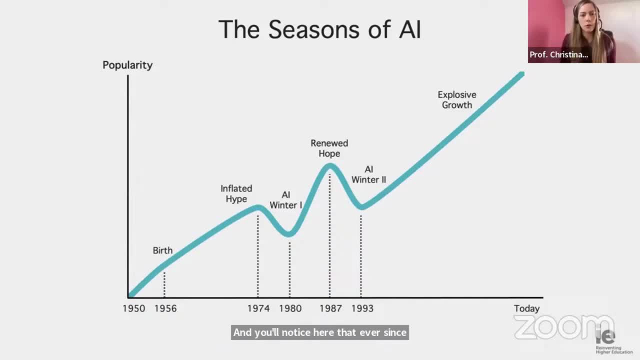 ever since then, we've been experiencing this explosive growth, that we haven't fallen back into an AI winter. Now, why is that? I'm going to give you a moment just to think on your own. Why do you think that we haven't fallen back into an AI winter yet? What is the difference? Why, since the early 90s, It just keeps growing. it just keeps going and going, and going. So I'll give you a moment to think. I'm going to share with you my hypothesis. 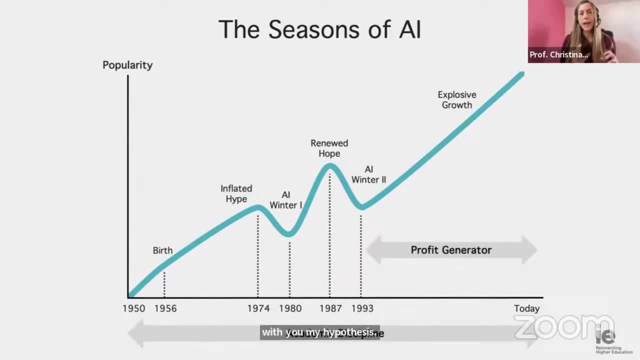 What I think has happened here is this: So AI began as an academic discipline and it still remains an academic discipline. It's very important in academia, But the difference here is that in the early 1990s it also started to become a profit generator. So it started to become used by companies, by businesses, and it started to bring value to these businesses for the first time. So it it expanded beyond academia And I think because of that we're seeing 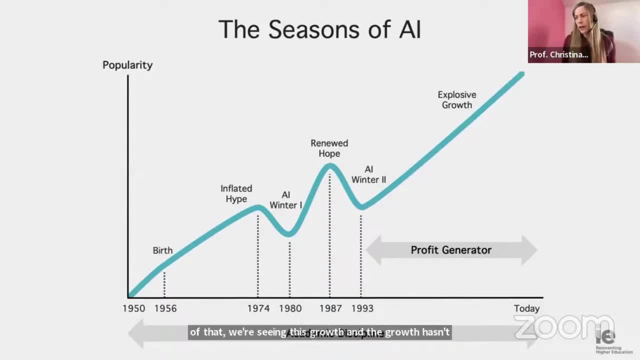 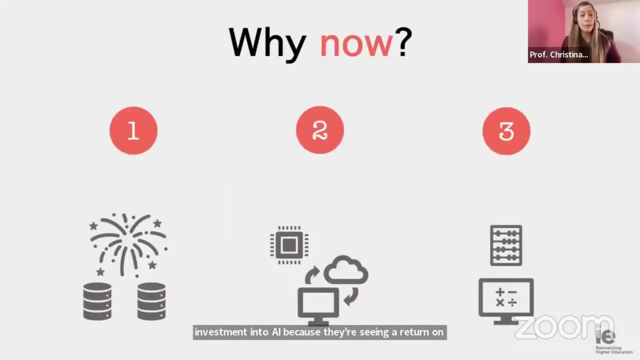 this growth and the growth hasn't slowed down. And you have to consider that with business, when there's money behind something, then things get done. So businesses keep throwing themselves and throwing investment into AI because they're seeing a return on this investment. Now this leads to what's happening today. So today especially, we are experiencing this huge growth in AI and explosion, And especially in the last, really the last couple years, this huge explosion. 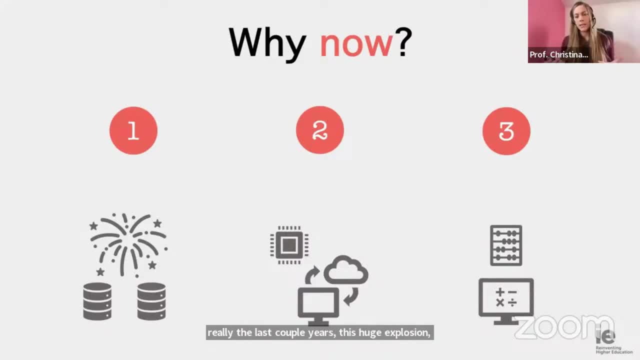 like a big data explosion. Why is that? So there's- I would say it's- the- the perfect storm, the perfect storm of three factors that have been brought together to allow AI to to take off like never before. So what is the first one? the first factor is this data explosion. So we've seen data growing and growing over the last decade. really, Why is it growing? It's it's the era of big data, And a lot of this has been. 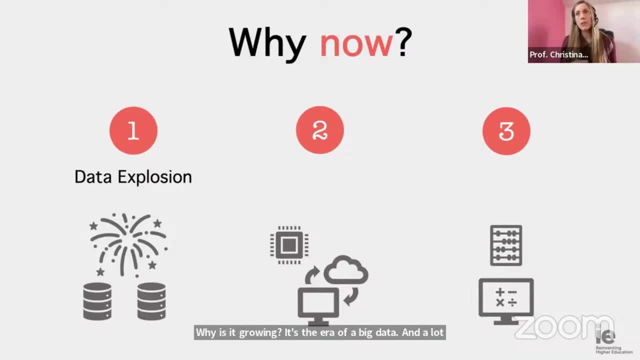 fueled by new types of data. So not only do we have more and more data, but we're also getting new types of data that we never had before. You have to consider, for example, that in the past, we typically worked with tables and spreadsheets of data databases, But over the last five years, 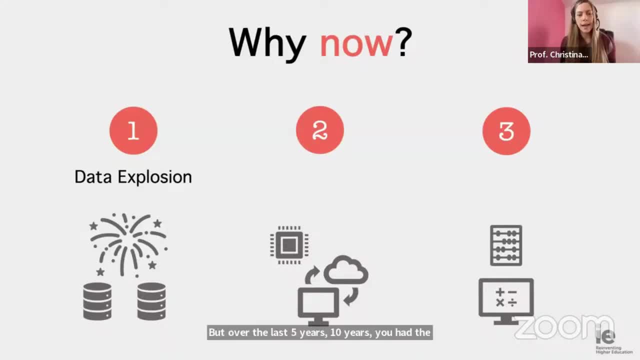 10 years you had the internet era exploding And now we're also adding new types of data, So data like photos and videos, music, GPS, all of these new types of data that are also being stored and analyzed, Data that we didn't have before and we also didn't have a way really to 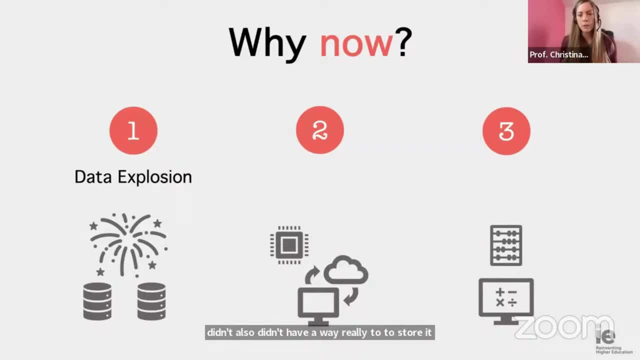 store it or to analyze it. But now we do So. we have these new types of data coming in, and it's a lot of data, not just human-generated data- We generate a lot of data- But as well now we have machine-generated data. So think about how much data is being produced by machines. 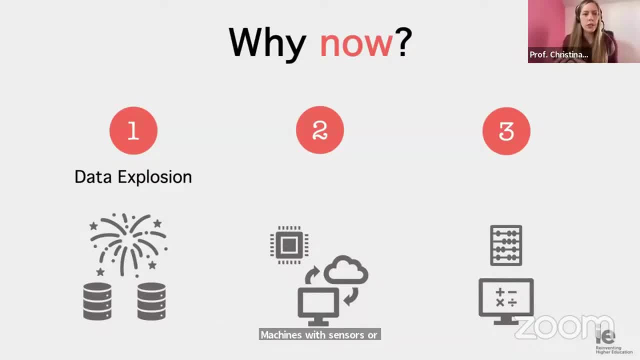 Machines with sensors or machines, whatever the data. your phone is collecting tons and tons of data and it's just growing and growing. So that's the data explosion. That's the first factor that I think has been contributing to this perfect storm for AI. Now the second factor is computing power. 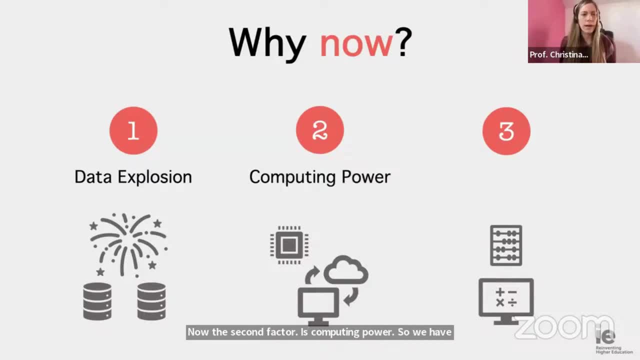 So we have more and we have cheaper computing power And there's a couple of different elements that fall into this. So one could be Moore's Law. If you're not familiar with Moore's Law, it's this idea that the transistors on a chip 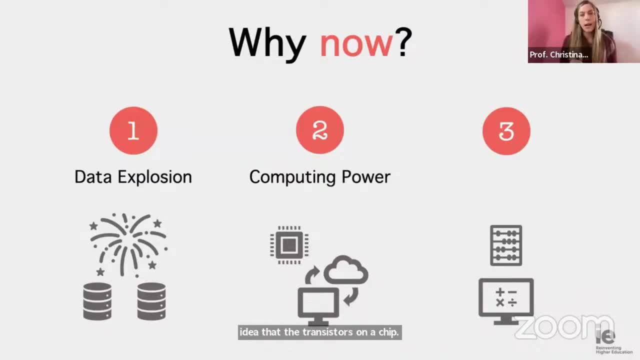 keep getting smaller and smaller, as well as cheaper, more affordable. So this whole idea of Moore's Law is what has allowed us to have our phones get smaller and smaller over time. You can imagine like 20 years ago or 25 years ago, phones were these massive, massive briefcases. 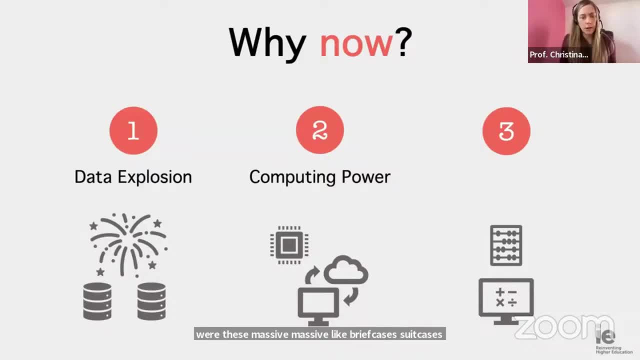 suitcases, And since then, the phones have gotten smaller and smaller, And so we've been smaller and smaller, And as well they've become more affordable, And all of this is because of Moore's Law As well. with computing power, another thing that's happening has been what I like to call 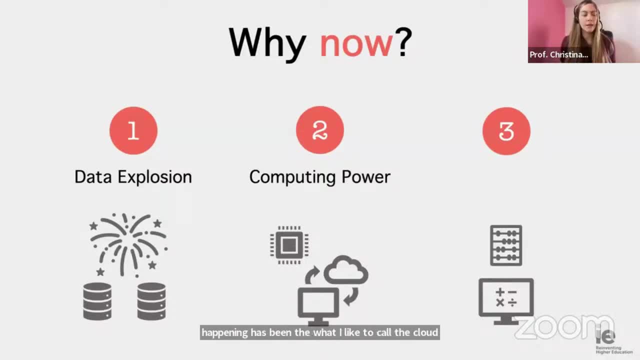 the cloud wars. So you have the cloud wars, particularly between Google Cloud, Amazon, AWS, Microsoft Azure- all of these tech players that are offering cloud solutions, And the cloud is really democratizing the use of data for everything, And so we've been seeing a lot of these. 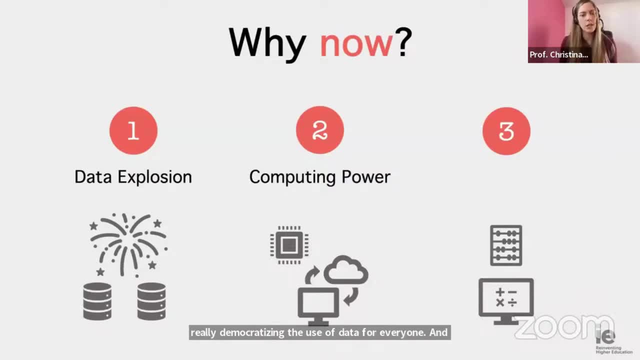 and not just data, but, of course, machine learning, artificial intelligence and so on. But it's allowing companies to more easily access the resources they need to create AI and machine learning products. And so you have, I said, Moore's Law, you have the. 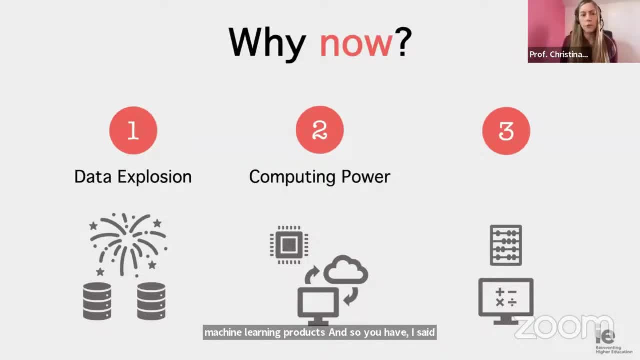 cloud wars. And then one last thing I would I would note here with computing power is as well this idea of AI, specialized processing units. So you have different processing units on machines. For example, a typical laptop computer would have a CPU, a central processing unit. 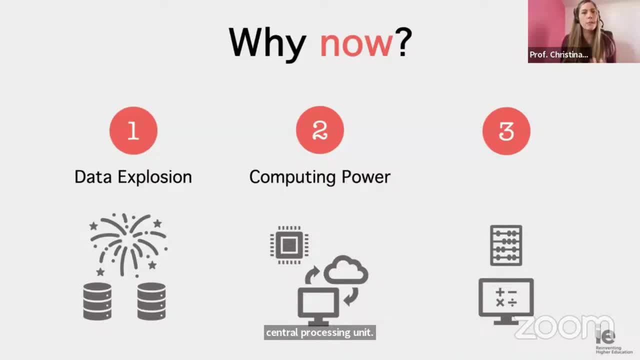 And these processing units. a CPU is great for the typical tasks that you want to do on your computer, But they're not so good at powering something as strong as an AI or training machine learning models. So what we've seen happen in the last years is companies are creating like 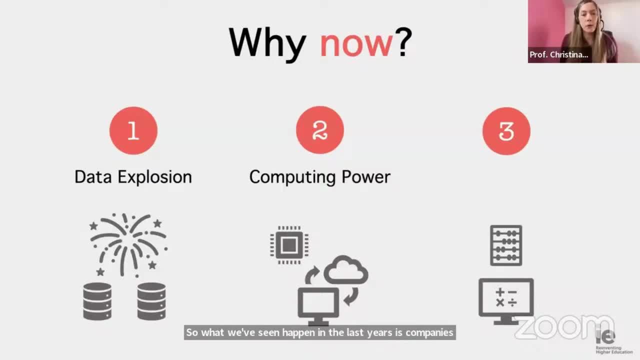 AI, specialized processing units to be able to power these machines, these models. You may have seen, for example, that NVIDIA, if you're familiar with NVIDIA- over the last- I think it was a few months ago- their stock started exploding. Their stock has. 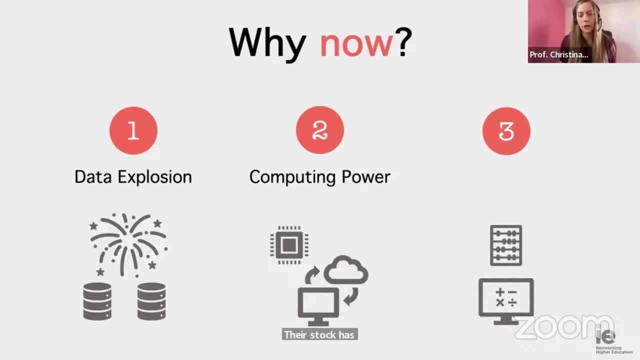 gone out of the roof. I mean, the value of the company has exploded. Why has this happened to NVIDIA? Because NVIDIA are the ones that are powering the era of AI right now. Why? Because NVIDIA? if you are a, if you are a video game player, then you're probably familiar with NVIDIA, because 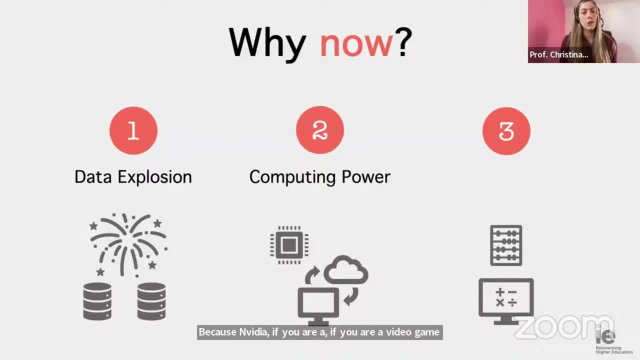 NVIDIA is well known for creating the GPU. It's called the graphics processing unit. This is a processing unit that is wonderful for graphics, which is great for video games, And they've been doing this for years. But what they found is that these graphic processing units 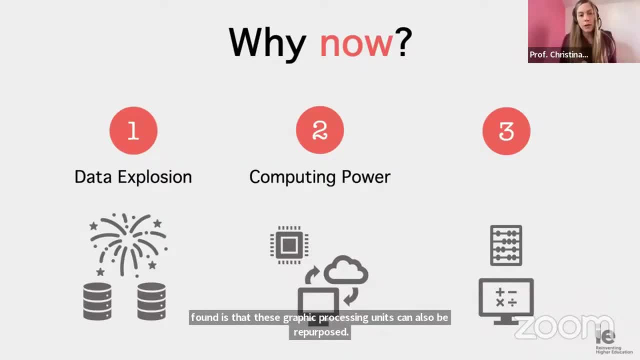 can also be repurposed. They're really powerful as well to power AI. So that's what's happened with NVIDIA. is that the is that their graphics processing units have been repurposed for AI, And that's why you've seen their stock blowing out of the roof. And then you 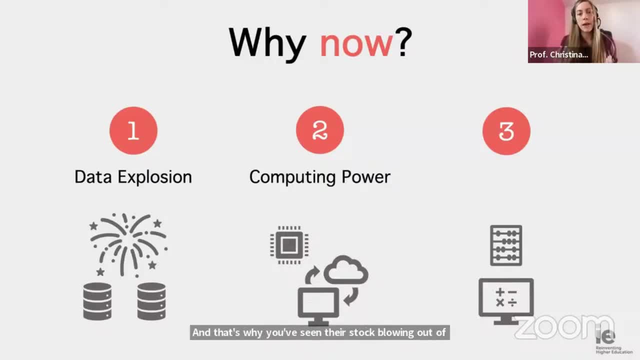 have, as well, a few other processing units by different companies that are being offered to help power AI. So that's the second, the second piece of the perfect storm. Now the third one is the fact that we have better algorithms. So better algorithms especially- you may have heard, 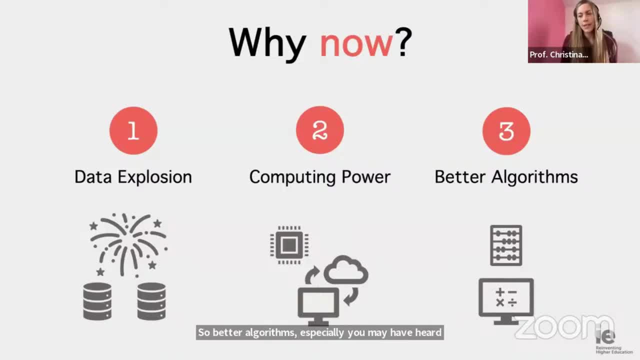 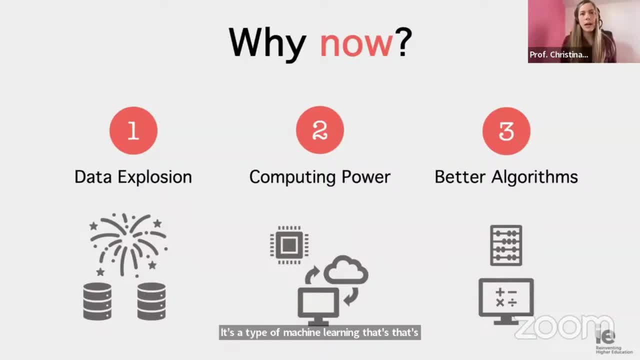 That's modeled after the human brain And it's very good at recognizing patterns and classifying things, So it's used in a lot of things around us today, And it's only been able to reach its full capacity recently because of the fact that we have the technology to power them. 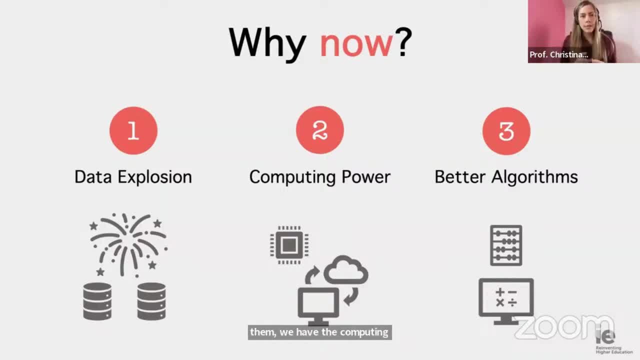 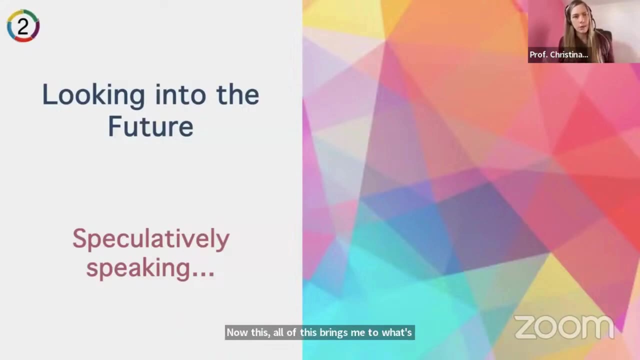 We have the computing power, we have the data. So you bring all of this together and now you've set the stage, you've set the foundation for AI to really start growing and exploding. Now this, all of this, brings me to what's happening today and also in the next years. 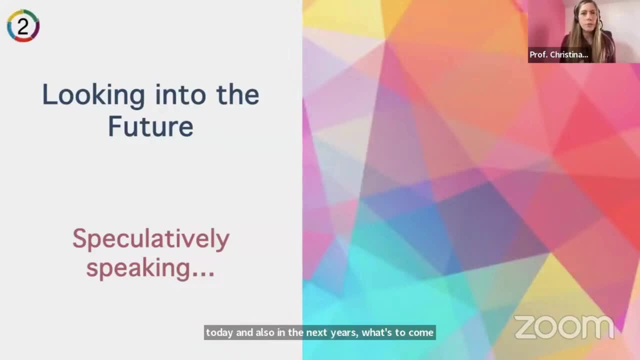 what's to come. So I wanted to make sure that I that I covered with you a little bit of my thoughts on what's happening now and looking into the future. What do we need? What do we need to keep top of mind? So the first thing that I wanted to highlight is that I think what's happening with AI, 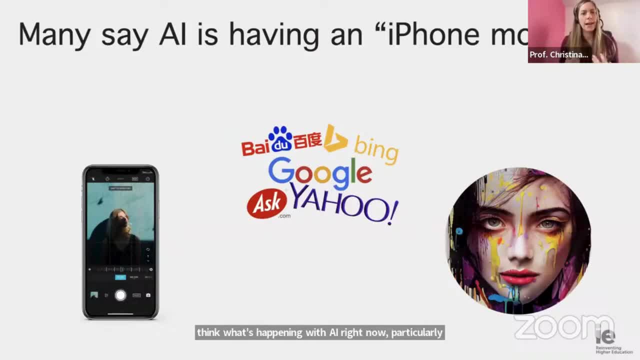 right now, particularly if we're talking about generative AI, chat, GBT, etc. I think what's happening right now with AI is that we're talking about a lot of things. that we're talking about. AI can be likened to two other relatively recent moments in history, So we could compare it to the 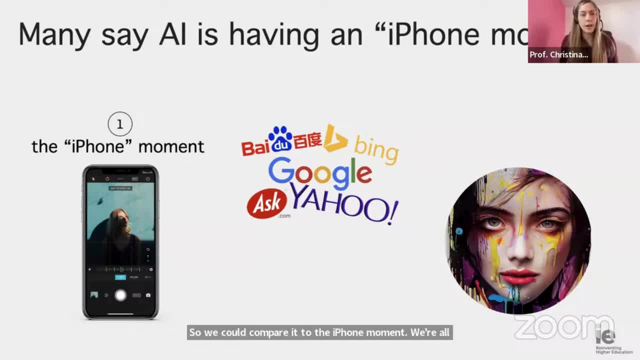 iPhone moment. We're all familiar with that, I think, when Steve Jobs came out with the iPhone announcement and all of us were in shock- this, this incredible device in our hand that could do so much. So we have the iPhone moment, And then as well. the second moment that I have here is the. 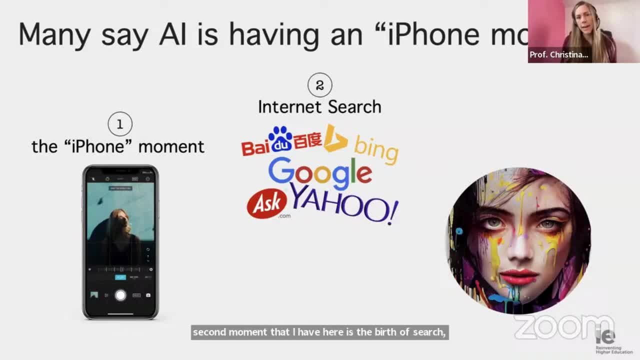 birth of search, of internet search. So I think what's happening now can be likened to these two moments. But the iPhone moment is more of like a technological, a technological advancement. So I think what's happening now can be best compared to internet search. That's the most. 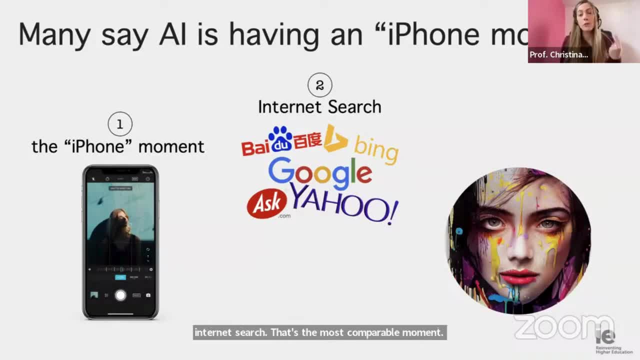 comparable moment. Internet search was actually the first wave of transformative AI. Now we're living through the second wave of transformative AI. So this first wave of transformative AI- internet search- this was all around ranking systems. So Google search is just a ranking algorithm. It's ranking all of the content on the internet. 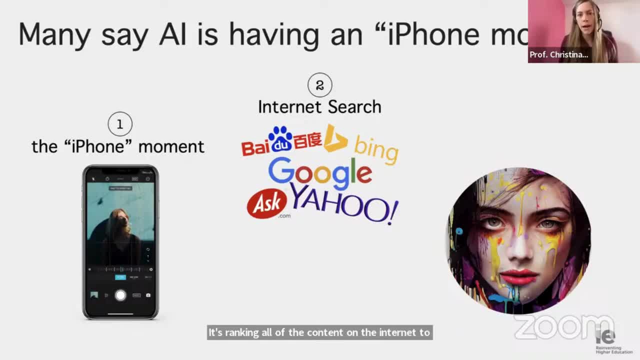 to decide what is the most relevant to show you, And this is the same idea that goes behind as well the recommendation algorithms, like on YouTube or Facebook, deciding what to show you. All of this goes back to ranking systems, And it sounds quite simple, but it's actually very. 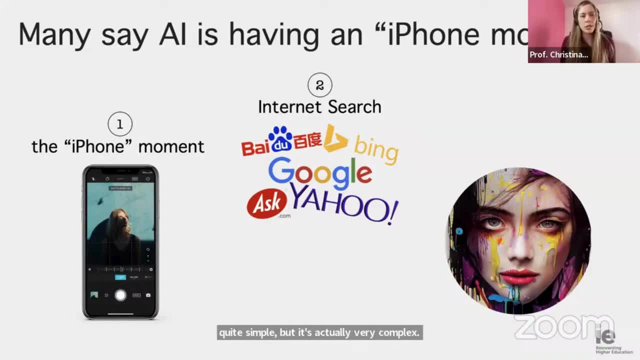 complex And as well. I think we've forgotten just how important this moment was. We've quickly gotten to the point where we're like: oh, we're going to do this, We're going to do this, We're going to do this. We've gotten used to having Google search at our fingertips And we've forgotten. 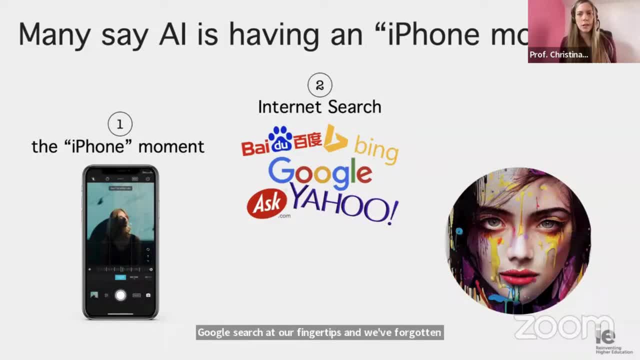 just how important that moment of history was. So this was the first moment, I think. Now what we're living through is this second wave of transformative AI, And this is the era of generative AI, And this is all about generating content. So remember, the first wave was about 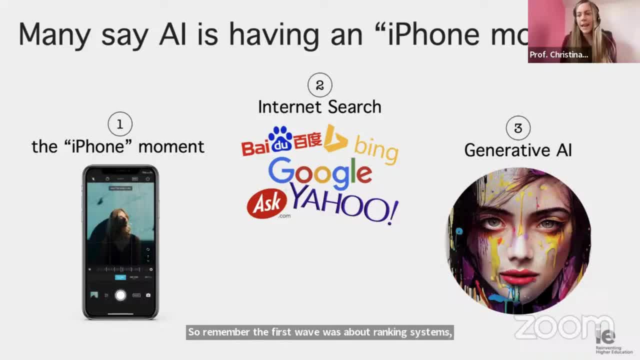 ranking systems, labeling and ranking things. Now we're doing something completely different, which is we have AI helping us generate new content, And this second wave has only just begun. We've really been living through it for just the past year, So this is the beginning. It's only a matter of time before we'll 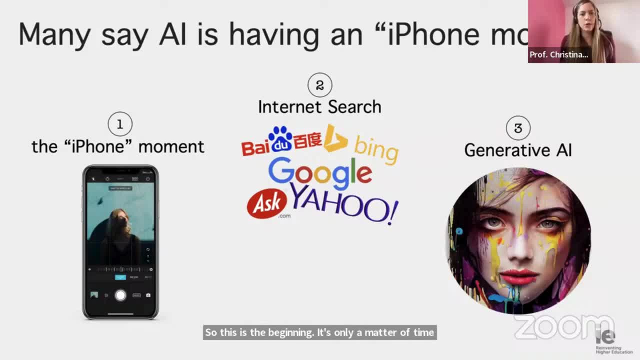 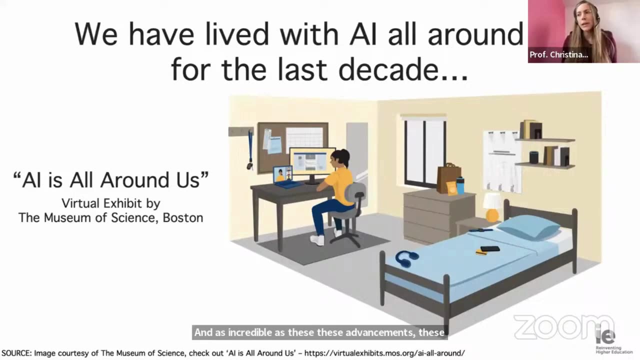 see how this might rewire our society. It's going to become a part of our everyday lives, the same way that Google search has become a part of our everyday lives. And as incredible as these recent advancements in AI are, I think we cannot forget that we've already been living with AI all. 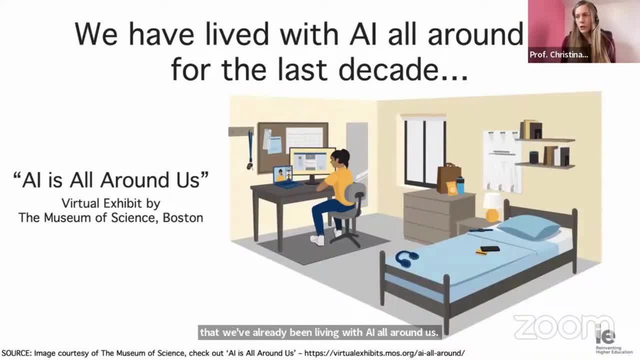 around us. So Google search is a good example, But there's also many other examples of ways that we are interacting with AI practically on a daily basis. So what I'm showing you here, this is from a virtual exhibit by the Museum of Science in Boston. This is from their website And, if you 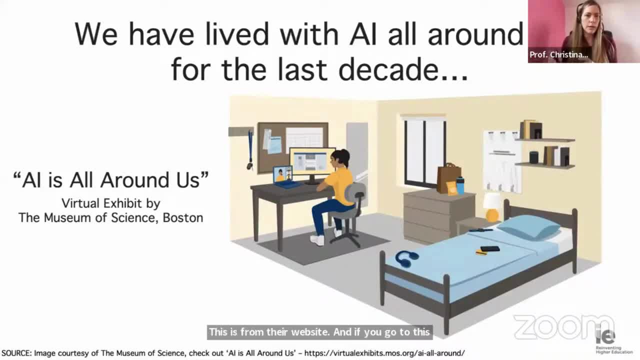 go to this page. it shows you what I'm showing you here. this picture, This is like a typical bedroom that they decided to show, And in the exhibit you can go and click different things in the image and it will tell you with each thing how is that connected back? 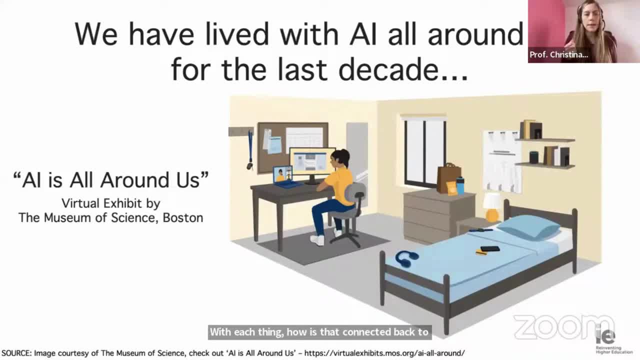 to AI Or how is that using AI? So, for example, maybe the headphones that you have, they might be using noise cancelling software that, in the end, is using AI to cancel out the noise. For example, as well, the smart speakers. So, if you have 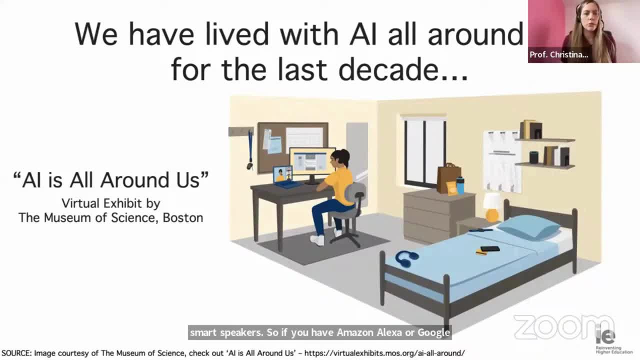 Amazon, Alexa or Google Home. these, of course, are using different forms of AI to work And many, many other things in the room, even if we consider, for example, the shopping- So you see the shopping bags on the table next to the bed. Even your shopping, most of the time, has been influenced. 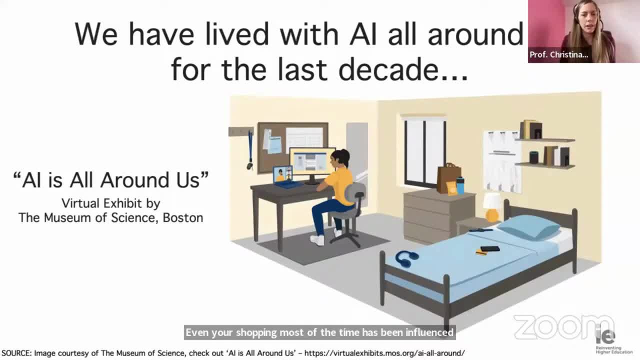 by AI. It's been influenced by the ads that you're seeing- online ads that are trying to convince you to go and buy different things. So as we start to look around the room, you'll find that a lot of things are in the room. So if you look in the room, you'll find that you'll be seeing a lot of things. 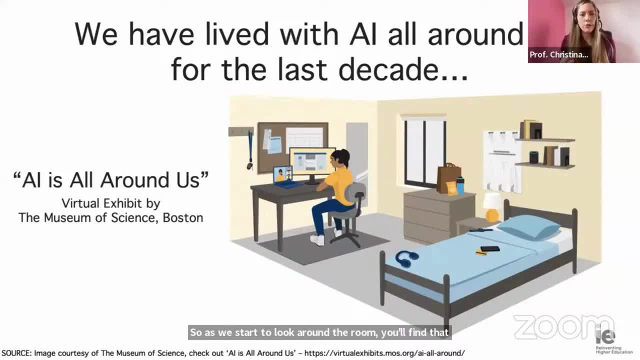 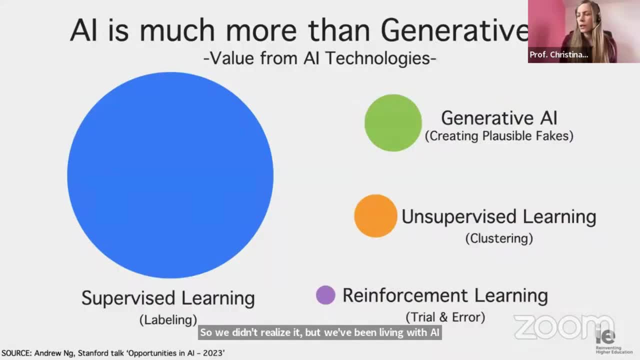 in some way or another, connect back to AI. So we didn't realize it, but we've been living with AI all around us, really for the last decade. Also, I wanted to highlight this point. This, I think, is very important. This is a point that I want to make sure that you're not blinded by all of 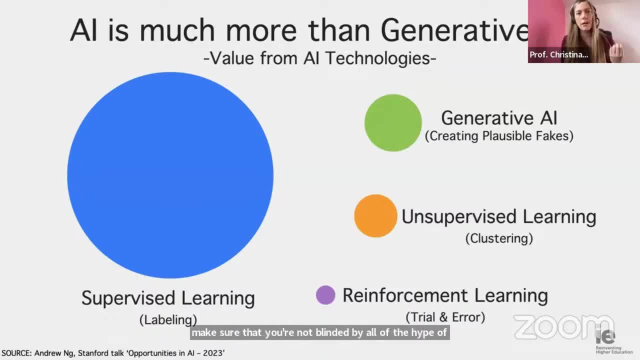 the hype of generative AI. So we're hearing a lot about generative AI right now- ChatGPT or tools like MidJourney that help you create new images And generative AI is incredible generating new content. but really the value of AI is not quite yet found in generative AI. Most of the AI 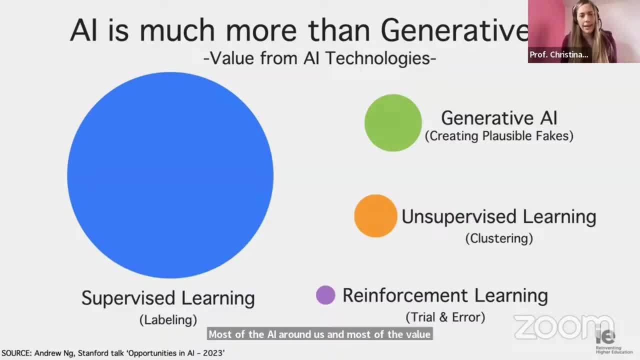 around us, and most of the value generated by AI is what we can call supervised learning, which is what you see here in blue. So think of most of the AI around us. it's supervised learning And, to put it in really simple terms, it's supervised learning. It's supervised learning. It's supervised learning. 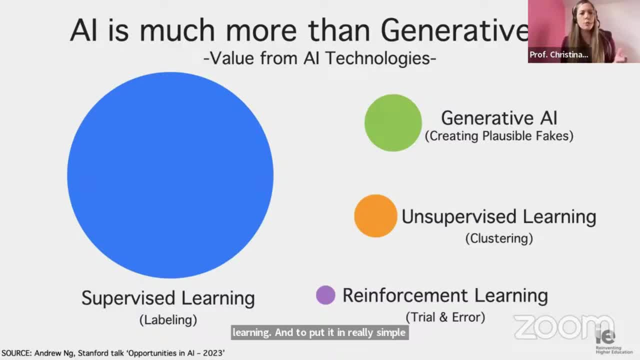 And, to put it in really simple terms, this is labeling, So labeling of content. This goes back as well to the internet search that I spoke about. That's really just labeling websites and any other sort of labeling, So imagine classifying of images. So when you go to 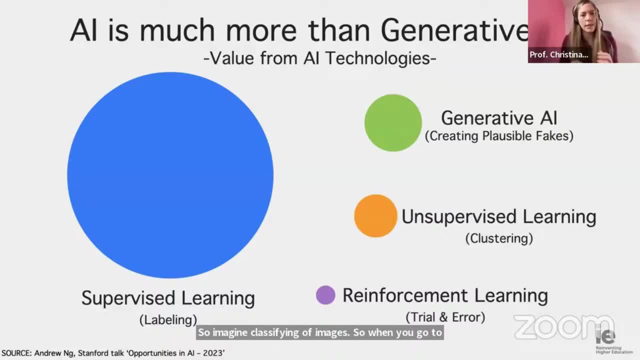 something like Google Image Search or any other website that lets you look at images. this has used supervised learning to label all of the content so that you can search for dogs versus cats. So supervised learning is most of the AI around us and it's also the most value. 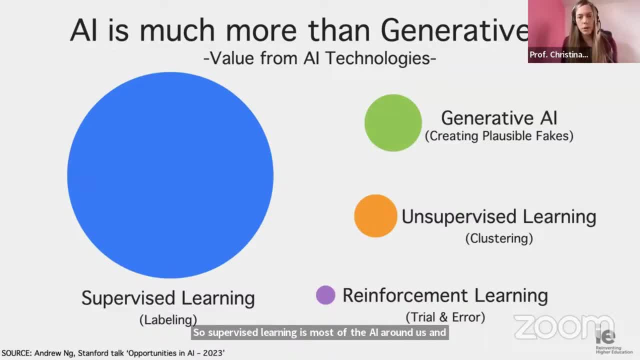 Then we have, in green, generative AI, which you should be familiar with, which is just think of, like ChatGPT, or even tools that help you create images or videos. That's generative AI. And then you also have here, as well, two other AIs that I wanted to highlight. 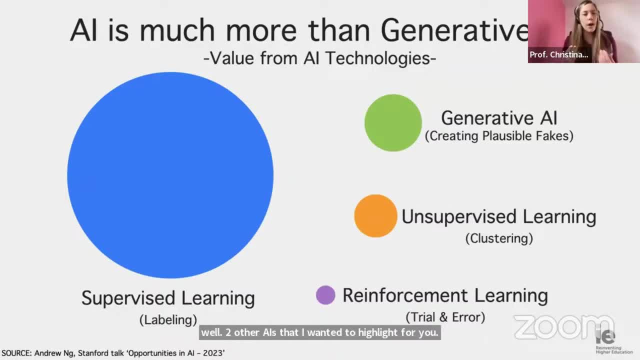 for you. So these are less used and they're not quite bringing as much value, but they're still important to know that they exist. So the first one is the one in orange that I have here, which is cluster learning, And this is clustering. So clustering- you can think of it's AI that helps. 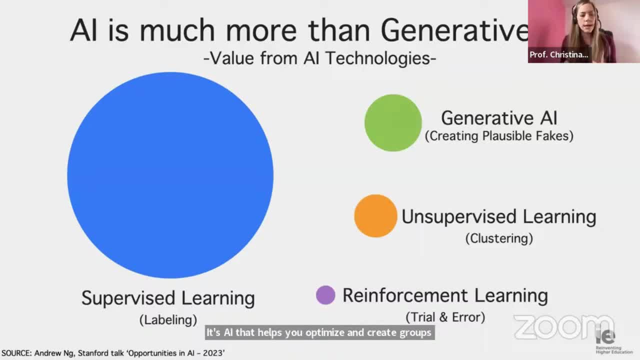 you optimize and create groups. A really simple example is to imagine like a retailer. So a retailer that has a big database of different clients and they want to build different groups of clients. Let's say they want to have five different groups that they can send specialized 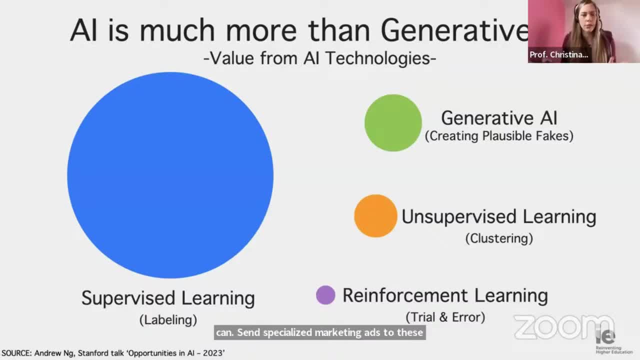 marketing ads to these groups, They can send them special deals. So the AI can help you optimize to create the best clusters: Clusters of groups that are similar within the cluster but different, different enough from the other clusters. So it's like an optimization task. And then the last one. 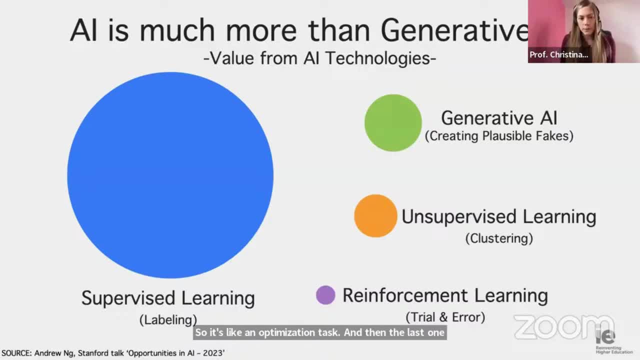 we have here, which is in purple, is reinforcement learning. So reinforcement learning, to me, I find it the most interesting type of AI, but it's the least used or least applicable today. And reinforcement learning- you can think of it like an AI that learns through trial and error. 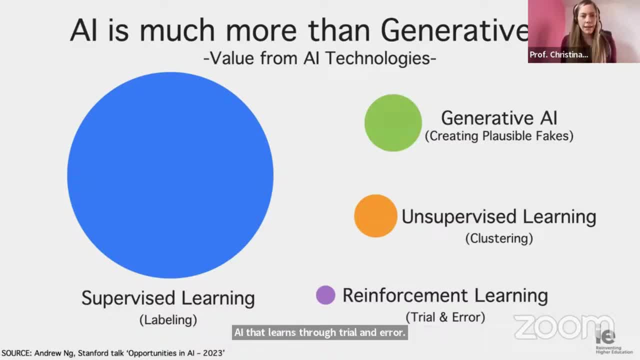 So, the same way that we often learn through trial and error, and AI can do the same. So imagine, for example, how a baby learns to walk. When a baby learns to walk, They learn through trial and error. They get up, they fall down, they get hurt, they learn from their mistake and they try to get. 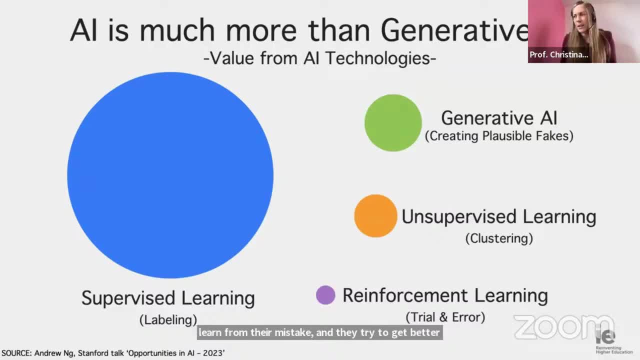 better and better just by trying it. So this is trial and error. the same- like a dog as well- that you train them to get a stick for you. if you throw a stick, you want the dog to bring it back. You can teach them through trial and error and they learn from their mistakes. So 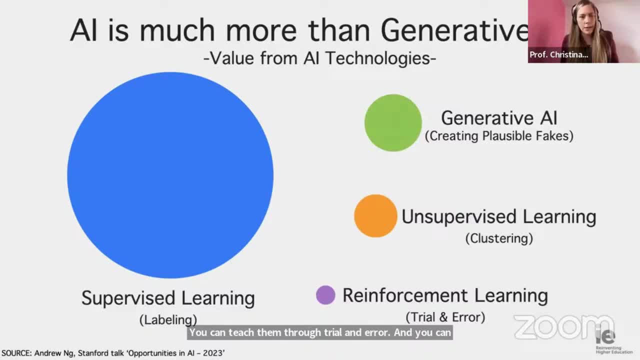 trial and error. you can give them rewards. you can give them a snack when they return with the stick so they learn through this what they're supposed to be doing. you can do the same thing with machines, and this is used a lot, particularly in robotics, to help with the movement, to learn how to walk. 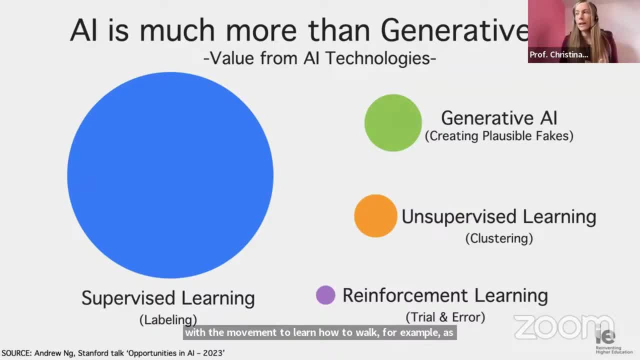 for example, as well, it's learned. it's used a lot in strategy. so, teaching a machine, for example, how to play chess or how to play checkers- whatever sort of strategy game, you can use this type of learning to train the AI to do that. so these are the four main types of AI and I want you to remember. 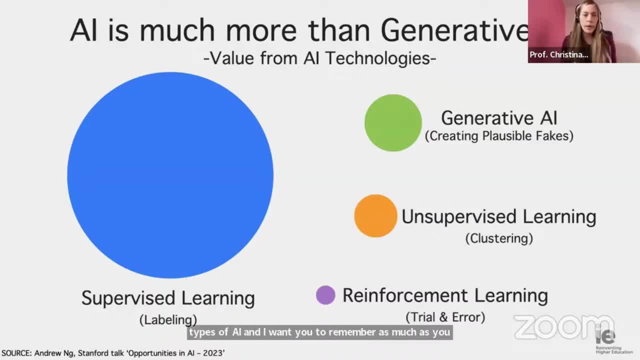 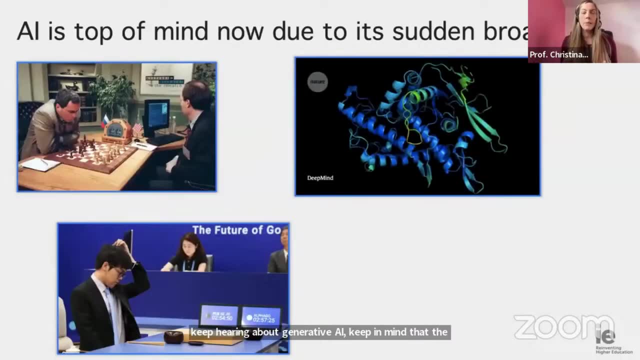 as much as you keep hearing about generative AI, keep in mind that the value and the use still remains in supervised learning here. one thing I did want to highlight, though, is that I know the generative AI doesn't have as much value you yet, or it's not used around us a lot, but the reason that we're hearing about it so much and the 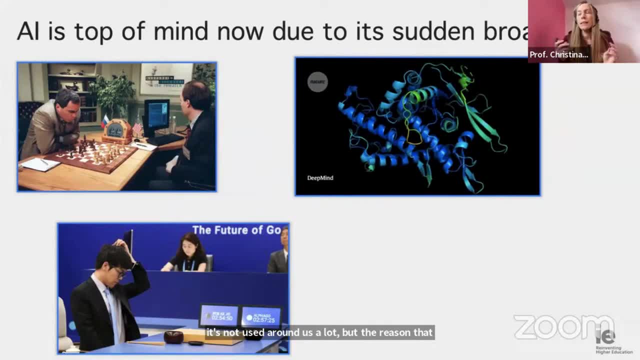 reason that it's making headlines is because this type of AI, generative AI, it's top of mind because of its sudden broad utility, and I'm going to explain that for you. the AI, this AI, generative AI, is very useful for everyone, so it actually has this broad utility that all of us can touch. 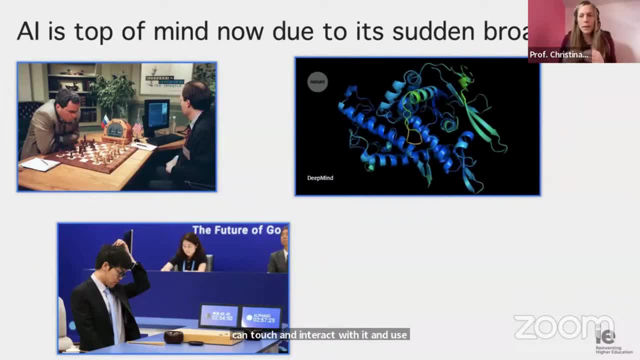 and interact with it and use it. but we've been, we've been developing AI for many years, have you, as you've seen? and there have been incredible, incredible moments and advancements in the field of AI. the only thing is that a lot of them, as incredible as they were, they didn't have this. 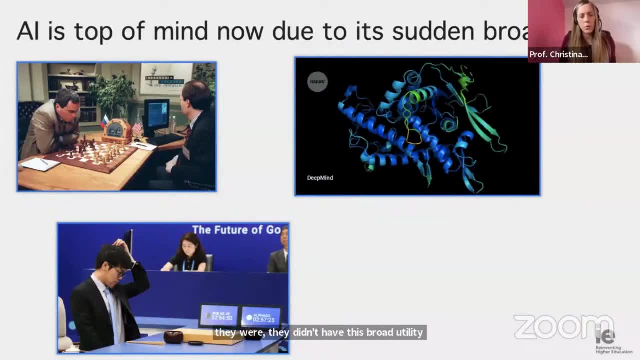 broad utility, like we couldn't interact with it. so we quickly forgot about it, and I'm going to show you a couple of examples here so you can understand what I mean. so the first example is in the top left, you see here. this is going back to 1996 when IBM's deep blue beat the world champion of chess, Gary Kasparov. so 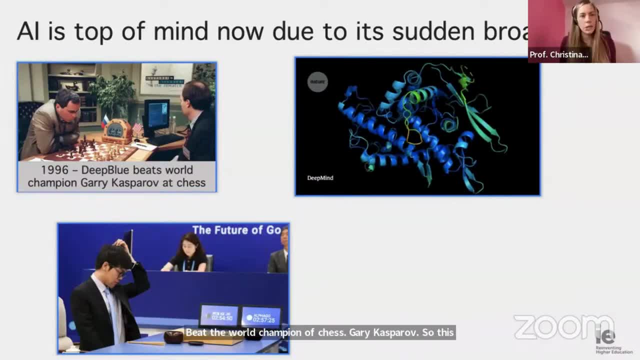 this is the first time that a machine beat the world champion in chess and at the moment this made all of the news. it was incredible, but we kind of forgot about it just because there's no broad utility for us. so, unless you're a chess player and you're playing with the machines, 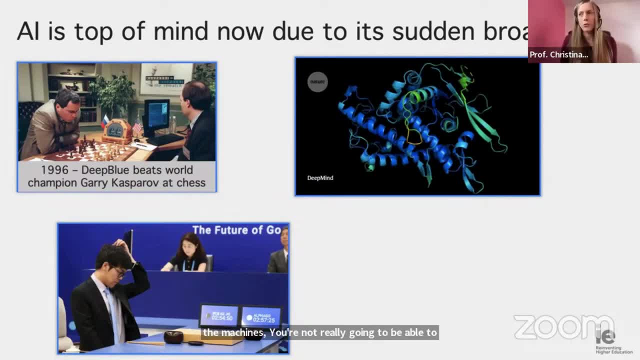 you're not really going to be able to interact with this much. so you read the news- it's incredible, and then we kind of forget about it. so that was one really important moment. another one happened. this was 20 years later, so you have the picture on the bottom. 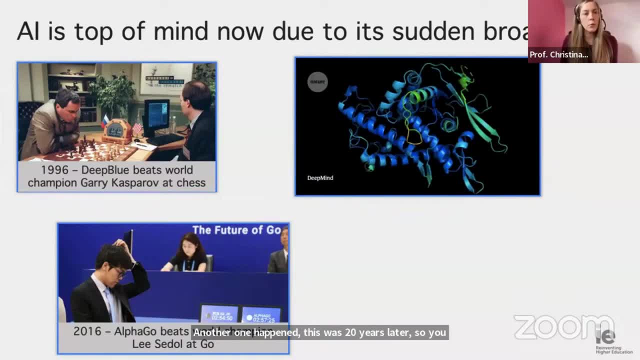 2016, AlphaGo beat the world champion Lee Sedol at Go. so Go is a Chinese strategy game that is supposed to be infinitely more complex than chess, and at the time, these champions of Go had said that it was impossible for a machine to beat the world champion of chess. and at the 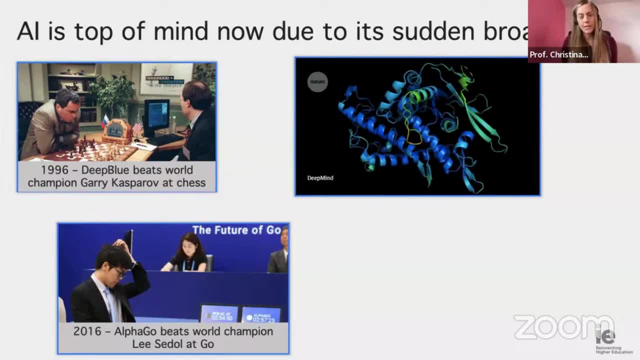 to beat the best players of Go, but they were wrong. in 2016 it happened. so, again, this was an incredible moment. it made a lot of headlines as well. there's a movie about it, I think it's called AlphaGo the movie- it's a documentary- highly recommended, by the way. it's really good. 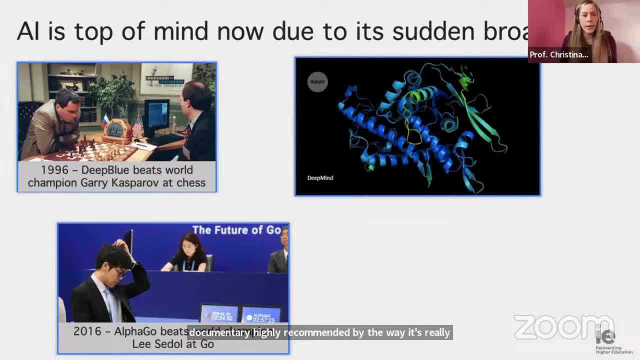 but this. so this happened and it was an incredible advancement. it was all over the news but again we forgot about it because we don't really interact with it. it's not so useful for us on a daily basis. So, Again, the last eingendium has been the most important moment since the advent of the two teams. Now the last ingendium's the most important one as well. it's a documentary that has been played over over four years. Apparently, there has been about ten years since it has been played over 24 hours, but again, we never got any of those days. 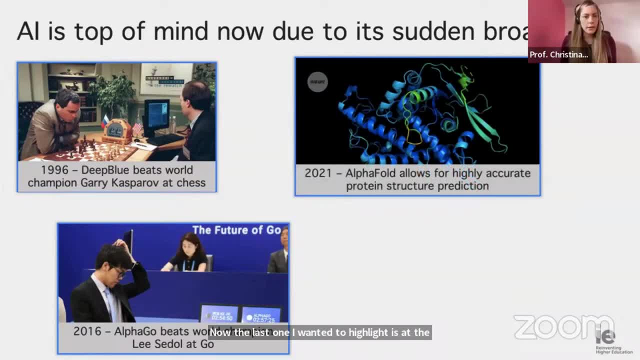 Also, it makes sense at that time. I wanted to highlight is at the top. This is five years later, in 2021.. AlphaFold allows for highly accurate protein structure prediction. So these were advancements, particularly in drug development and biology, that now we can use AI to help us create these new protein structures. And again, 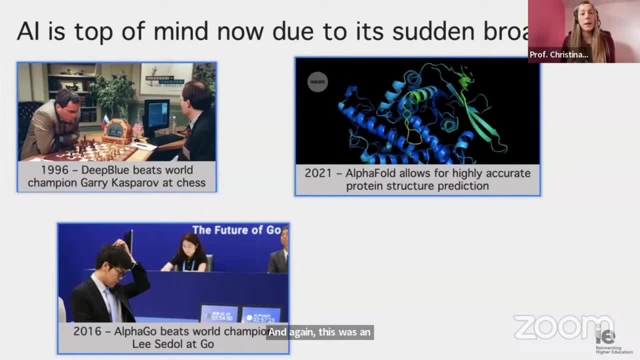 this was an incredible advancement in the field of AI, But unless you're a biologist or a drug, you're working in drug development. it's not very useful for you, So you don't have a way to touch or interact with it and you quickly forget about this. So all of these moments, 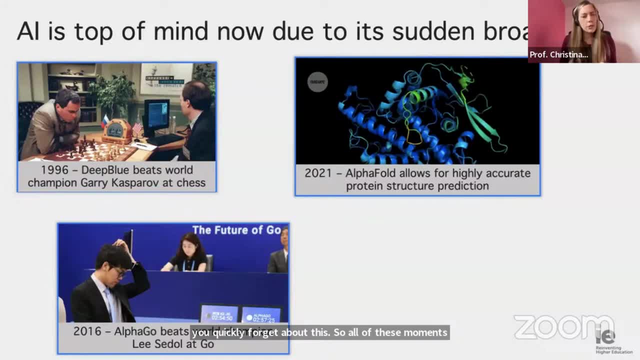 as incredible as they were, they were very useful for a specific part of the population, but not for everyone. Nowadays, though, with the advent of ChatGPT, stable diffusion, mid-journey, etc- all of these tools- we can actually use them to be more productive on the job. 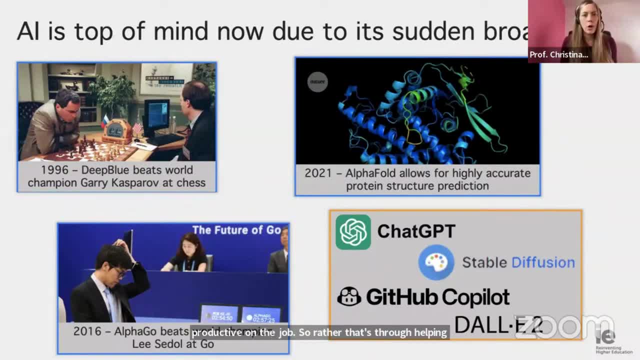 So, whether that's through helping us with writing, with coding, with pictures and videos, but for the first time now we're seeing this AI that we can use. all of us can use it. We can use it on a daily basis and it can help us with a wide variety of different work tasks. So I think 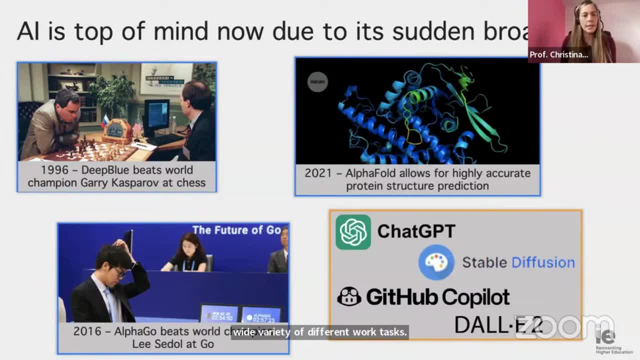 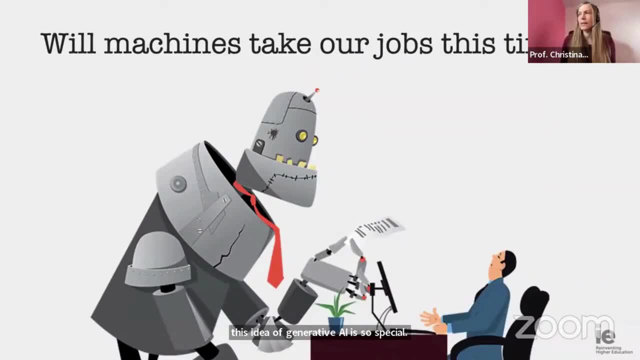 that's why we have it so top of mind and why this idea of generative AI is so special. Now, one question I get a lot in my classes and in talks is people always ask me: okay, but the machines, are they going to take our jobs this time? Now, remember. 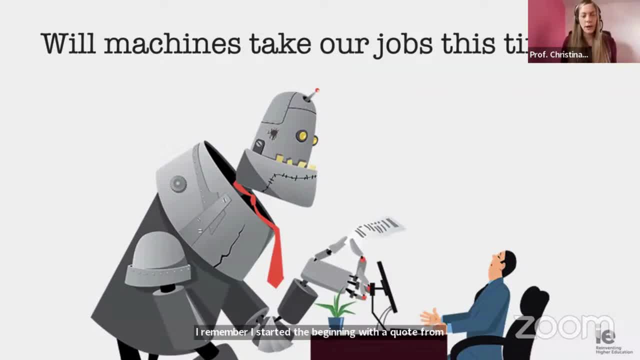 I started the beginning with a quote from Pedro Domingos about how the machines are not going to take our jobs, but we do need to learn how to use the technology, or someone else might learn and take our job. So I don't think the machines themselves are here to take our jobs this time. 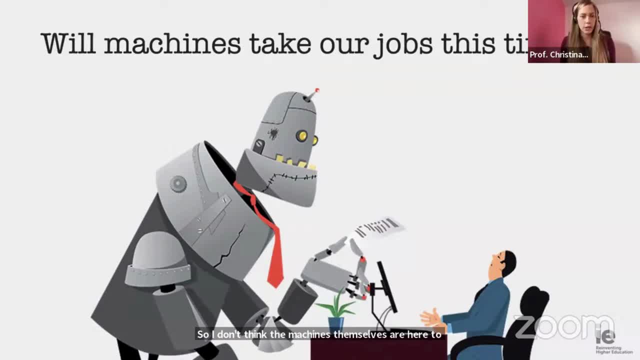 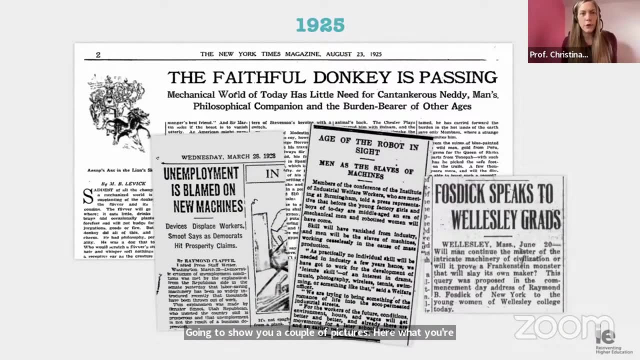 And this is not the first time that we've asked ourselves this question. I'm going to show you a newspaper from 1925.. And you can see it says: unemployment is blamed on new machines, an age of the robot in sight, men as the slaves of machines. So this was 1925. We're talking about 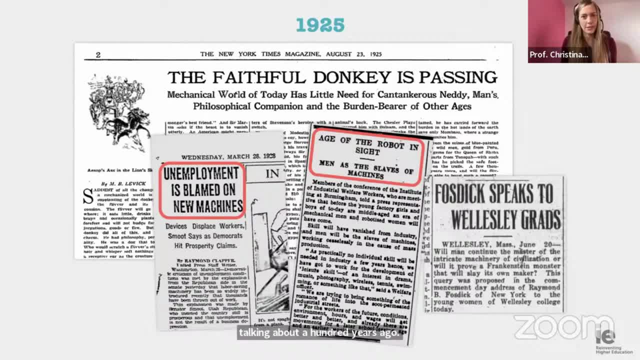 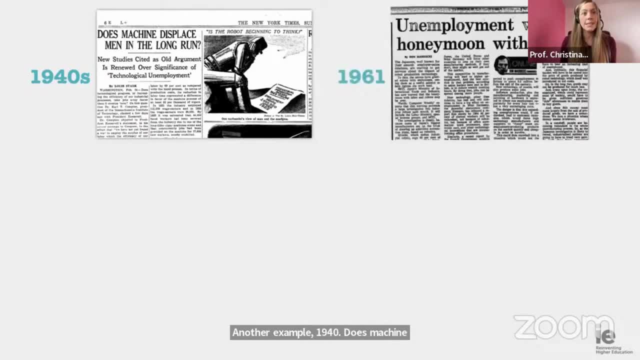 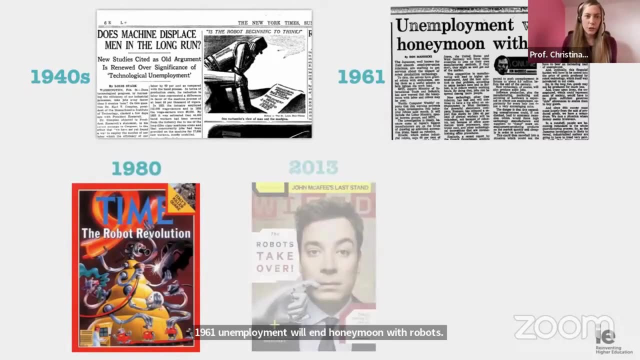 100 years ago, we were already asking ourselves these questions. Another example: 1940s: does machine displace men in the long run? 1961, unemployment will end. honeymoon with robots. 1980, the robot revolution. 2013, the robots take over. And finally 2017,. 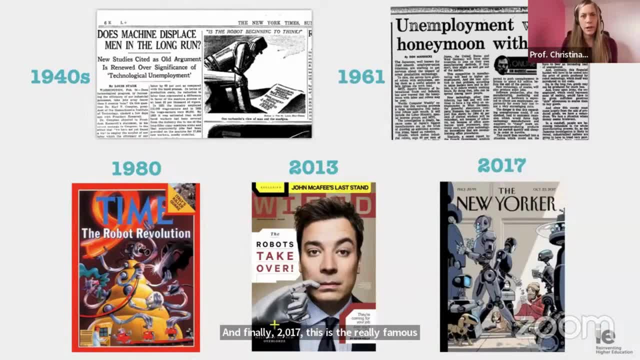 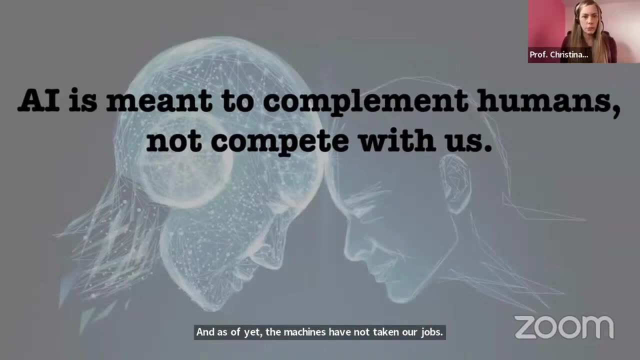 this is a really famous cover from the New Yorker. So you can see here we've been asking ourselves this question over and over for the past 100 years And as of yet the machines have not taken our jobs. The machines and AI is specifically meant to complement humans. It's not meant to. 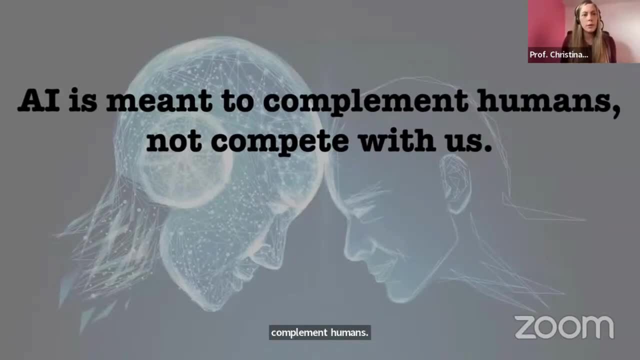 compete with us. It's true that some jobs will be semi-partly automated, Some of them might even be fully automated, But most of the time, these jobs what happens is new jobs are created And what we have to do is retrain the parts of the population that are affected. But we've never 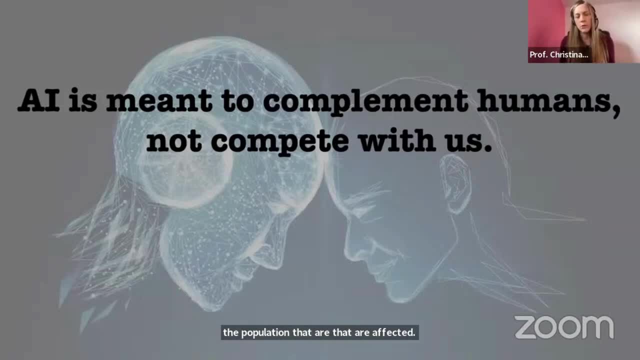 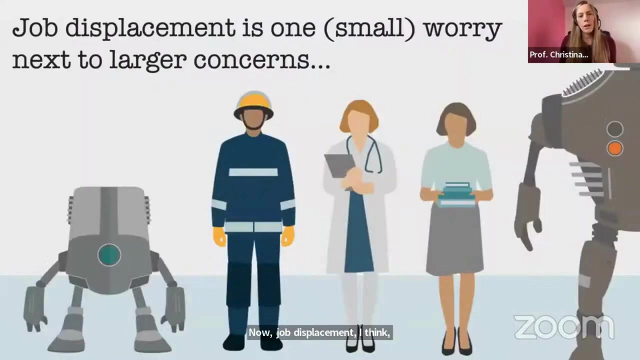 lived through a huge, dramatic moment. We've always been able to adapt to the changes And, in most cases, what AI is doing is it's meant to complement or empower you. The job displacement, I think, is one very small worry next to larger concerns, So I wanted to 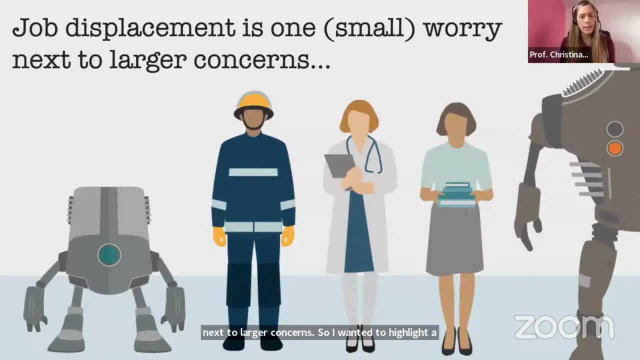 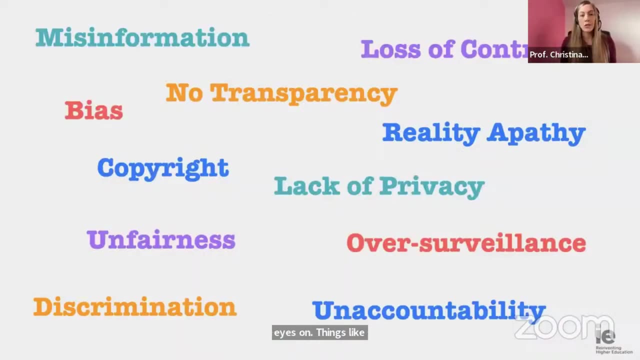 highlight a couple of concerns that we should keep top of mind in the years to come, Because I think job displacement is not something that we should be so concerned with. But there are a few things that we should be keeping our eyes on, Things like misinformation, bias, discrimination. 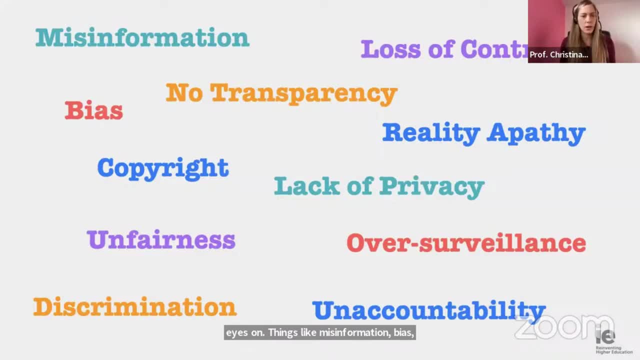 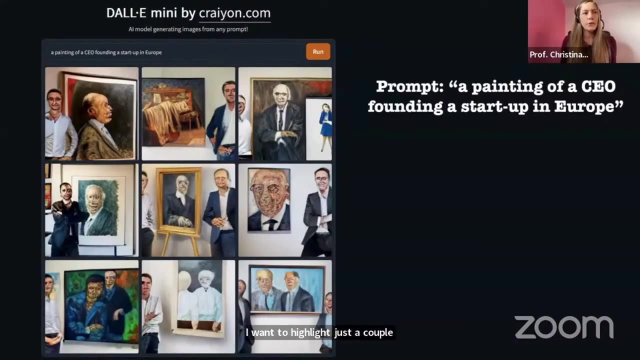 copyright transparency and so on. So all of these types of ideas, these are challenging And these are more short-term concerns that we need to keep top of mind. I'm going to highlight just a couple examples, a couple of examples here before we finish. So this first one, this example. 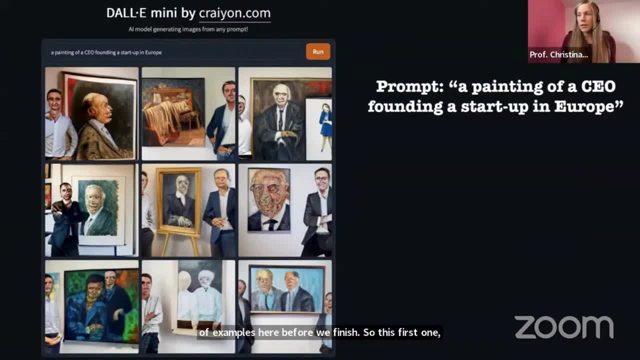 I'm showing you is from. this is using DALI. DALI is one of these generative AI tools that creates images for you. This was done quite a few months ago- And I'm going to show you a couple of examples here as well- And it was using a prompt. The prompt was a painting of a CEO founding a startup. 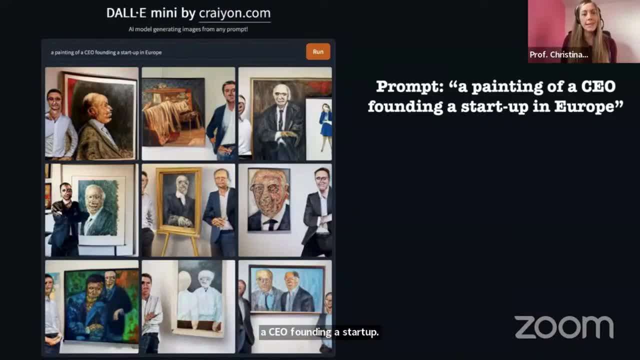 in Europe. So what's strange about these nine images that the AI produced for me? For me, I asked myself where are the women? And not just where are the women, but where is the diversity? In all of the images, it's the same type of person displayed: It's a white, middle-aged male. 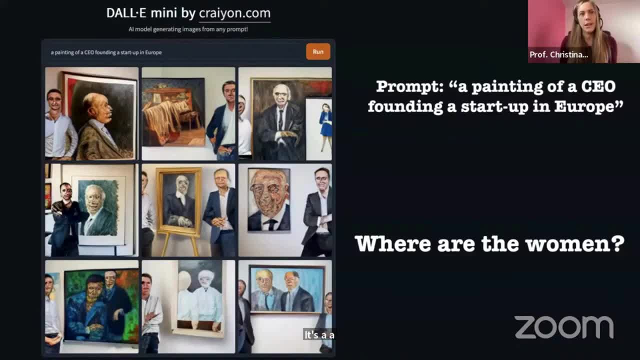 for example. So there's no, There's no diversity here, And this tends to happen. This goes back to discrimination and bias in our algorithms. Now, I told you that this was done quite a few months ago, When all of these tools launched ChatGPT and then the other ones for images like MidJourney DALI, when they 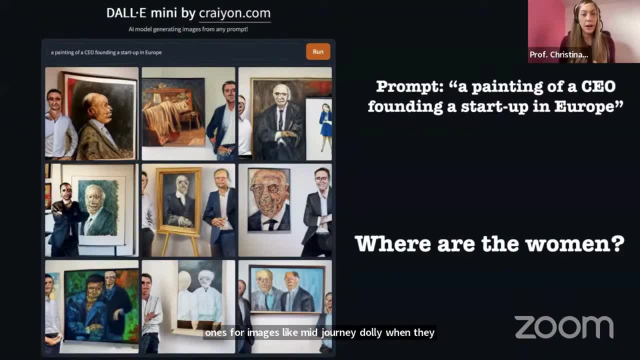 launched. they were launched, actually, with a lot of bias, a lot of bias in their responses, things like this, And they've been working on improving them over time and trying to introduce more diversity, Because what they were doing is they were proliferating a lot of discrimination and bias. 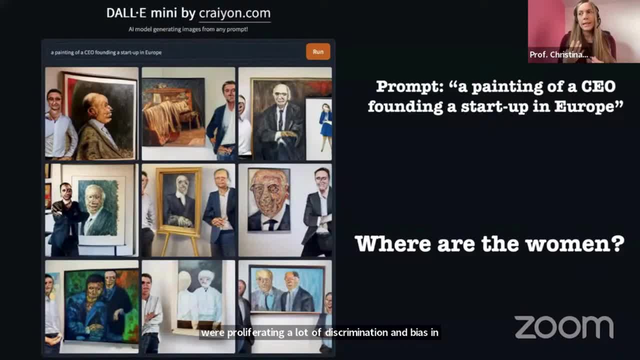 in their output. Why does this happen? It's because of the data that we're training it on. So I think I've mentioned a few times with you all today, but you have to remember that AI is fed by data. So it's the nutrition for the AI, is the data that you're feeding it, And it learns from this. 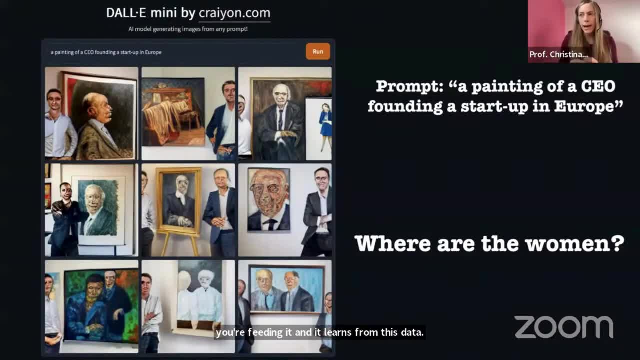 data And, for example, in this case, if we train the AI with a lot of historical data of CEOs in Europe, if a lot of those CEOs have the same, if they're the same person, if it's all a middle age white male, for example, then the AI is just going to repeat that pattern into the future. It. 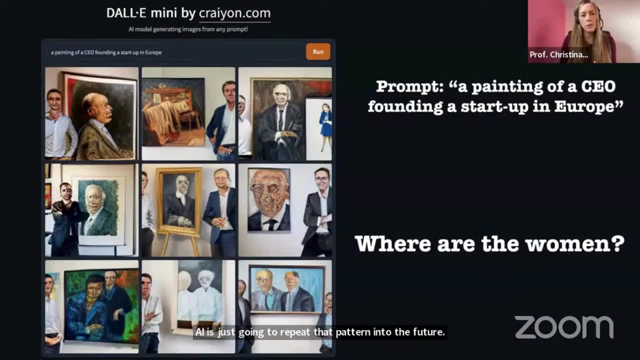 doesn't know any better than what, than the data that it's seen. So we have to remember that we need to try to use diverse data sets. we need to introduce diversity into that training phase to help the AI have a more diverse perspective of the world. So this is one example I wanted. 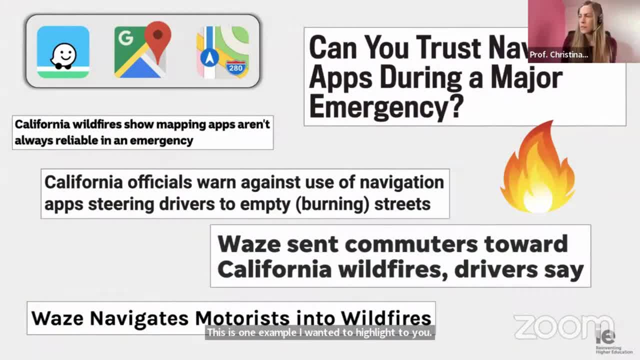 to highlight to you Another one. This happened a couple years ago with Waze. So in California, in the US, California has these really big, dangerous wildfires And it was found that people were going to Waze to try to leave the wildfire And Waze was directing them to go straight. 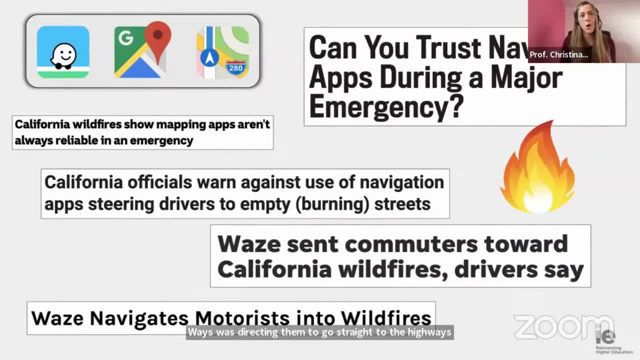 to the highways that were engulfed in flames. Why was Waze doing this? Waze was doing this because Waze was built to avoid traffic, So all of these highways that were covered in fire- obviously there was no traffic on the highway, So Waze was leading people directly to these dangerous paths, And this is 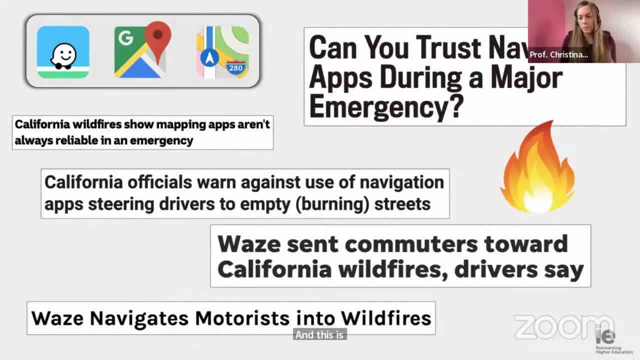 because, again, this goes back to what I was saying before, that the AI is trained on. you know what you train it to do. So in this case, if Waze is trained to avoid traffic and nothing else, then that's all it's going to do. It doesn't have a view, an outside view of the world. It doesn't have. 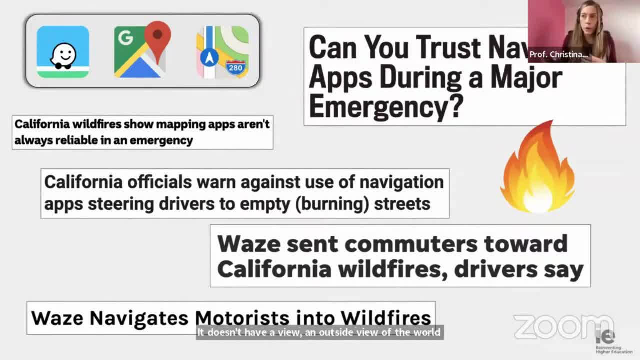 a world around it. It doesn't understand the world like we do. So if you want Waze to also avoid fires or natural disasters, then you have to train the AI to do that. You have to give it more data about the world so it can understand that it needs to optimize for these points as well. 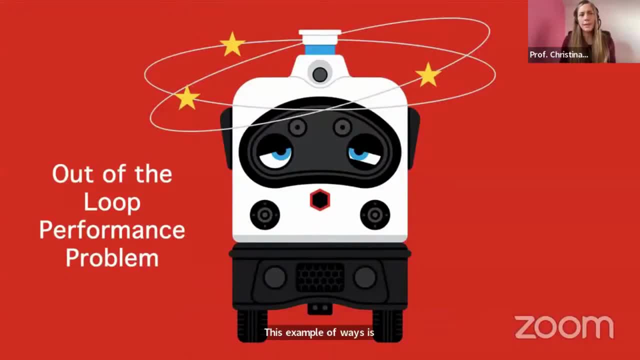 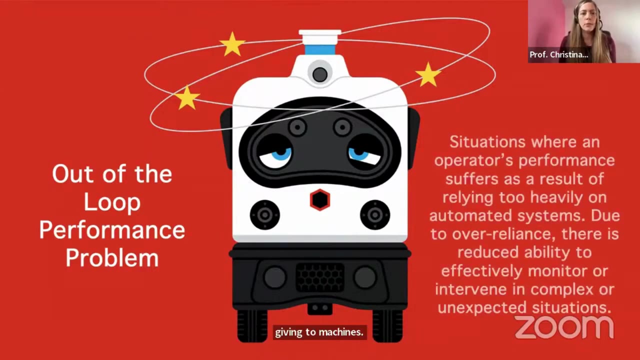 This example of Waze is actually what we call the out-of-the-loop performance problem, And we're experiencing this a lot and a lot more now because of how much power we're giving to machines. We're a little bit of control. So this out-of-the-loop performance problem, it's situations where an 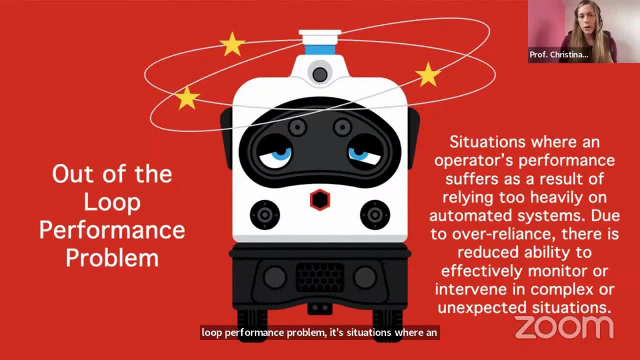 operator's performance suffers as a result of relying too heavily on automated systems. Due to over-reliance, there is reduced ability to effectively monitor or intervene in complex or unexpected situations. So this is exactly what happened with Waze- that we kind of lose control. 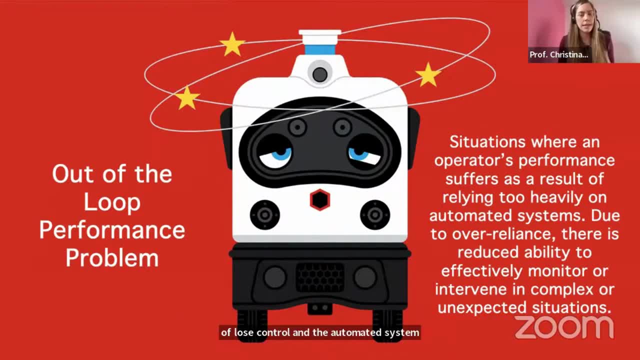 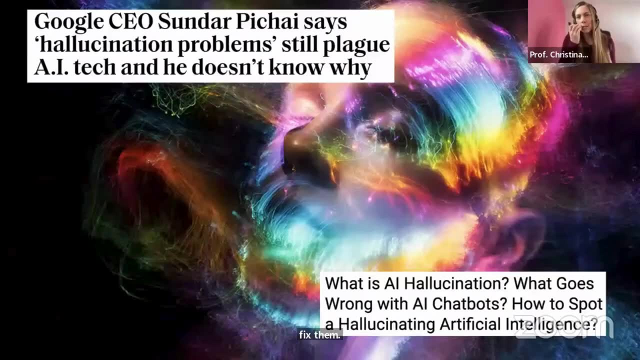 and the automated system starts to make mistakes, And it's very hard to control the system, So we're going to go back and fix them. It takes some time. And a last couple of things that I wanted to show you as well. This is referring to the hallucination problem that a lot of the AIs are having today. You 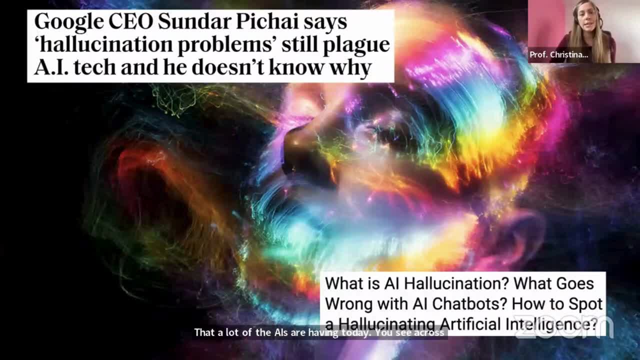 see across the top. Google's Sundar Pichai says hallucination problems still plague AI tech And he doesn't know why Hallucinations is when a tool like Chajibiti. it can lie, So Chajibiti can lie. 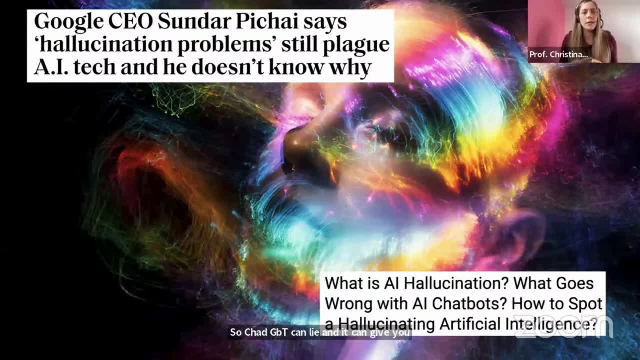 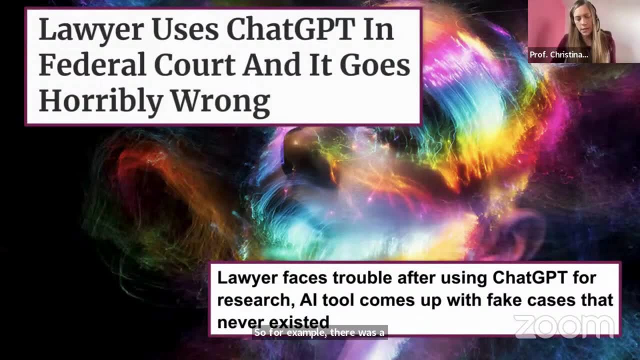 to you. It can give you answers, It sounds very confident, but it can completely fabricate the answers. So, for example, there was a lawyer months ago in the US that got in big trouble because the lawyer was using Chajibiti to prepare for trial And Chajibiti was giving him false cases. 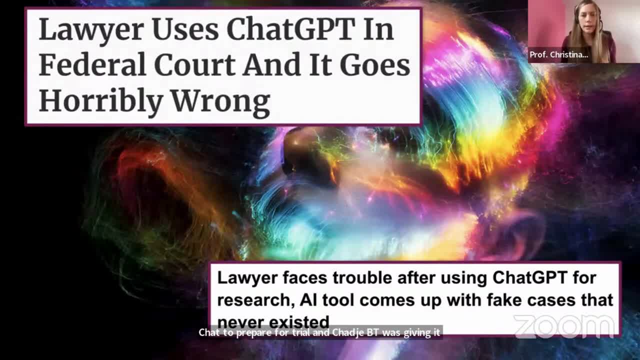 And the lawyer went and presented in court false, fabricated cases from Chajibiti, Obviously got into a lot of trouble, But the lawyer didn't realize that Chajibiti can lie. Chajibiti can create things. So keep in mind that AI can hallucinate and it can fabricate lies. 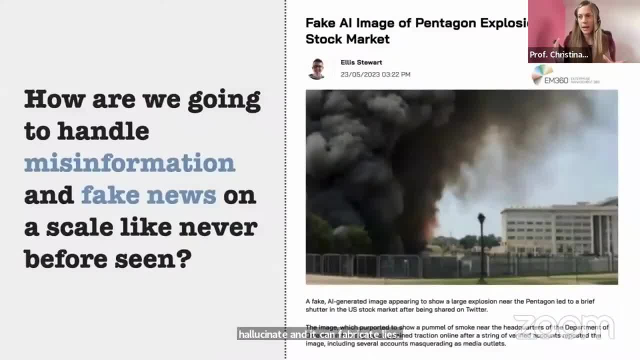 And the last thing that I wanted to, one other problem that I wanted to highlight for you to really get the wheels turning in your head as well: How are we going to handle misinformation and fake news on a scale like never before seen? What you're seeing in the image here. 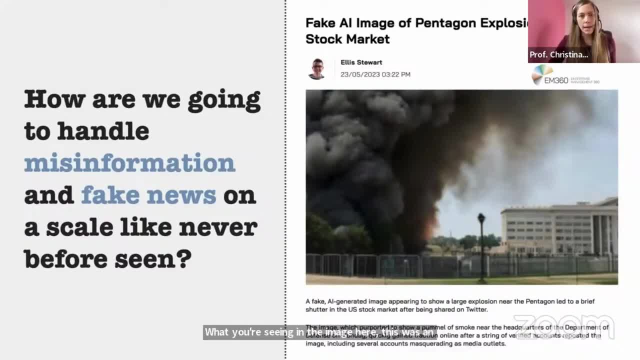 this was an AI generated image. This was back in May. It's a little bit younger now And I started creating it last year. We just released the Sawmall picture video a While ago- a veryuite And, as you can see, this AI generated image was supposed to be showing an. 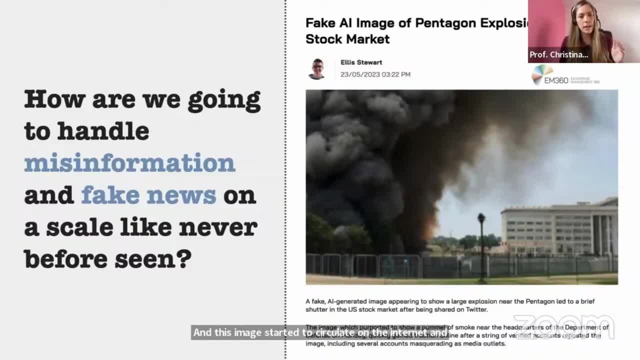 explosion at the Pentagon in the US And this image started to circulate on the Internet And it also caused the stock market to fall down a little bit. The stock market fell a little bit before people realized that the image was fake. So we have to be very careful now with misinformation and fake news. 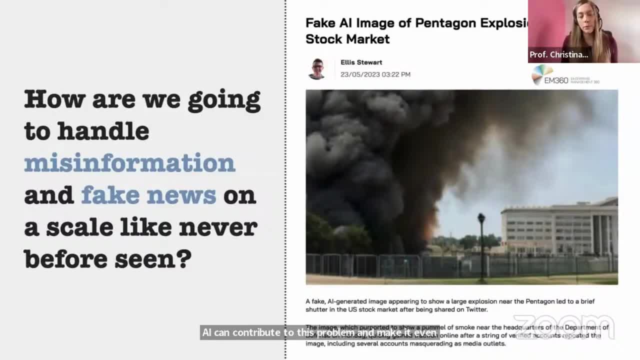 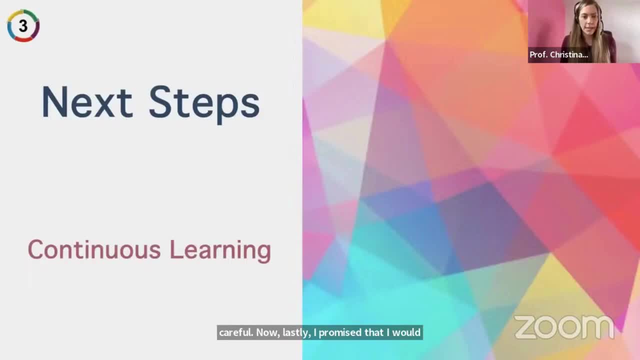 AI can contribute to this problem and make it even harder to tell what's real from fake. we have to keep this in mind and be careful Now. lastly, I promised that I would close with a couple of next steps, So I wanted to leave you with recommendations If you want to keep learning. 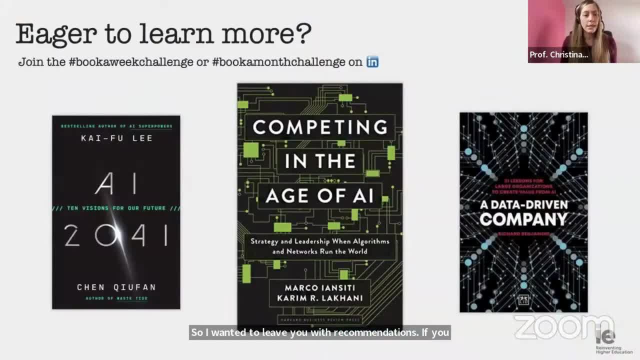 about this subject, then I highly recommend these three books, So feel free as well. if you want to take a screenshot right now, you're more than welcome to- But these are three books that I recommend you check out if you want to keep learning. AI 2041 on the far left- this is more. 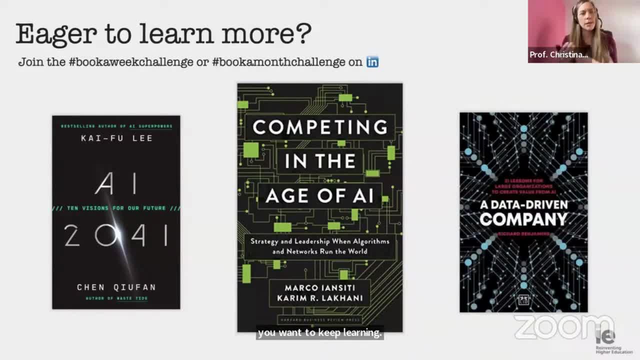 like futuristic 10 visions for our future with AI. It's a very like entertaining book. None of these are technical, by the way. anybody can read them and understand The one in the middle: competing in the age of AI. This is about really business and strategy. How do you keep competing now in 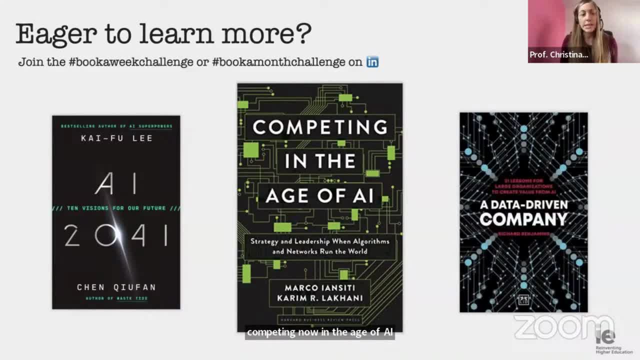 the age of AI. And then the last one on the right is a data driven company. Actually, I have it right here: A data driven company. This is 21 lessons for large organizations to create value from AI, And it goes back to having a data first strategy And it goes through what you need to do to do that. 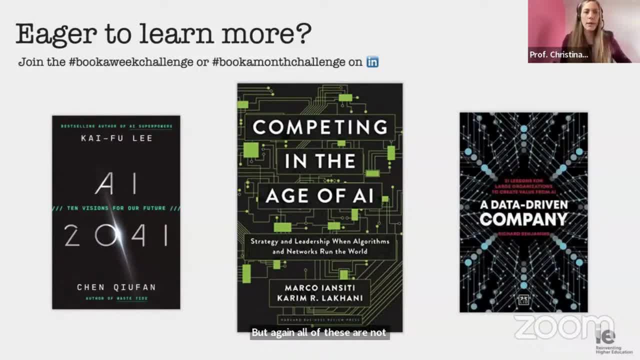 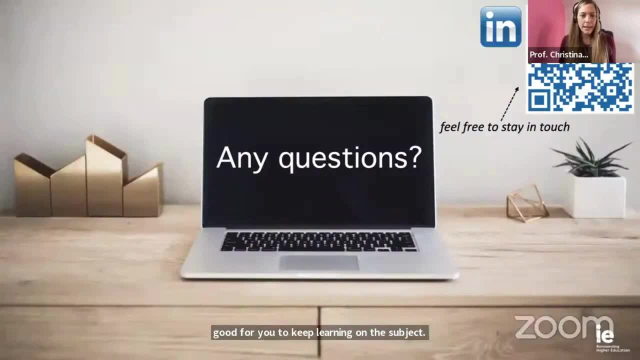 But again, all of these are not technical. They are written for audiences from any background And they're good for you to keep learning on the subject. So that is everything from me. I wanted to welcome you. feel free, you can. you can scan the QR code here if you'd like to stay in touch over. 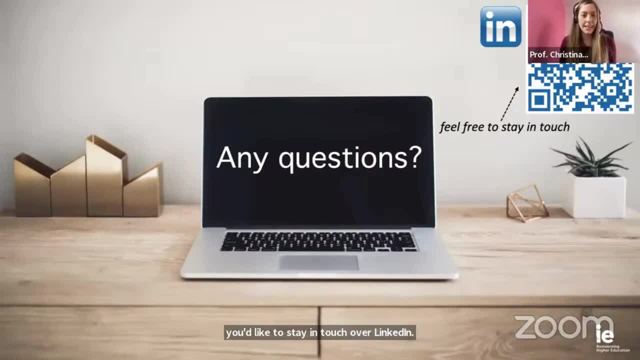 LinkedIn, I share daily content on all things data and AI And I'm I'm happy to open the floor. I don't know if we're going to do questions now. we might have a little bit from questions now or IE, but perfect, Okay, I'm gonna. I'm gonna hand the stage to Namita. 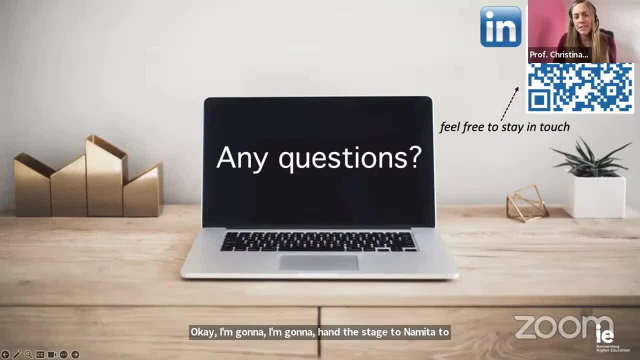 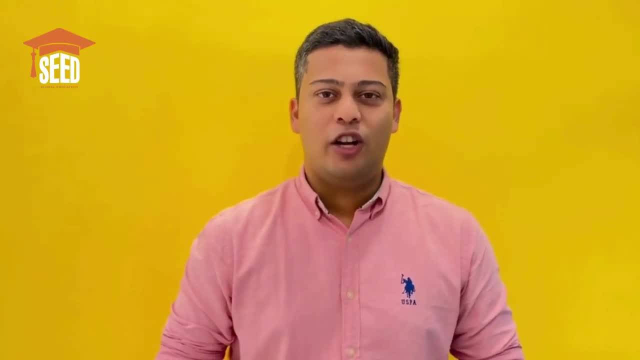 to talk to you about IE, And then we're going to be able to address any of the questions that you might have. Thank you so much for joining us.